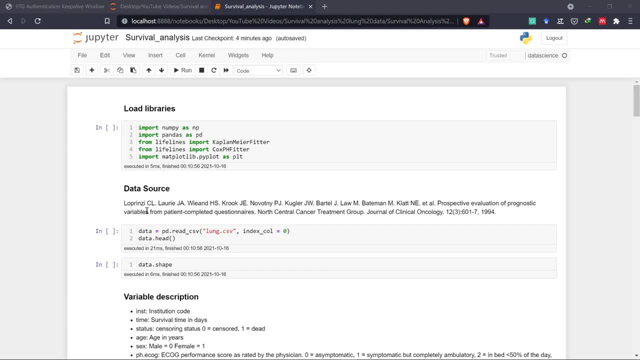 take leverage of and make decisions. if they know that the battery will die after three year, then state-wise, wherever the purchase rates are high for that model, they can allocate this kind of batteries there so that the consumer can buy it, which is very convenient, or go to that as a shop and easily get that even. 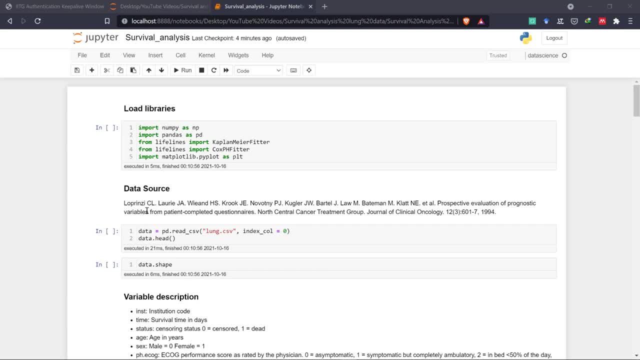 i mean transportation engineer. so in transportation research we can also leverage this for, say, pedestrian research. if a pedestrian arriving at an intersection and if the phase for pedestrian signal is red, so what would be the waiting time after that, the pedestrian say and will: there is no willingness for that. 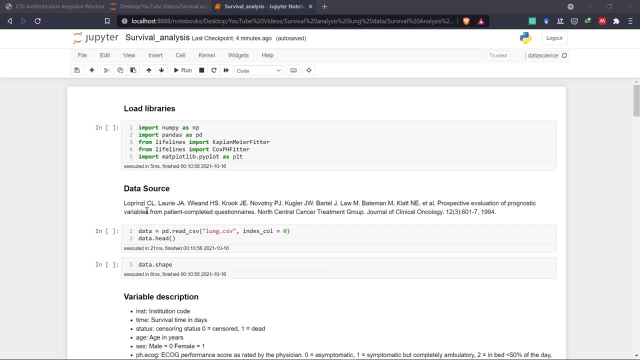 petition to wait more, or or he or she violates that signal. so when the pedestrian is lost, loses such patience actually. so, in aggregate manner, we can use this time to event analysis to identify what is the probability that the pedestrian waits for 50 second, or what is the time up to which 50 percent of the pedestrian 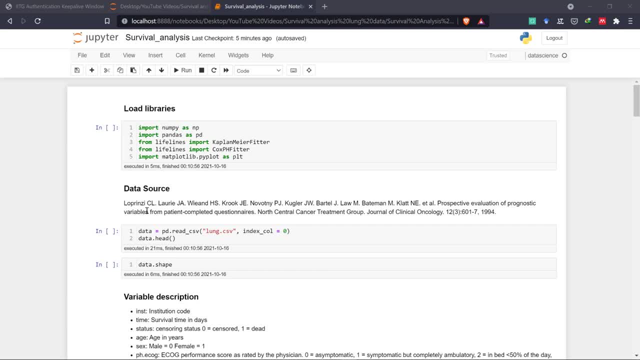 stays or wait for the green for this kind of time analysis. we can use this time to event analysis. that was used for, say, vaccine research or checking the effectiveness of medicine, uh like risk. it's also used in, say, uh vaccine treatments, like for current coronavirus treatment. say, a company comes up with a random selection of uh, say a control group and a. 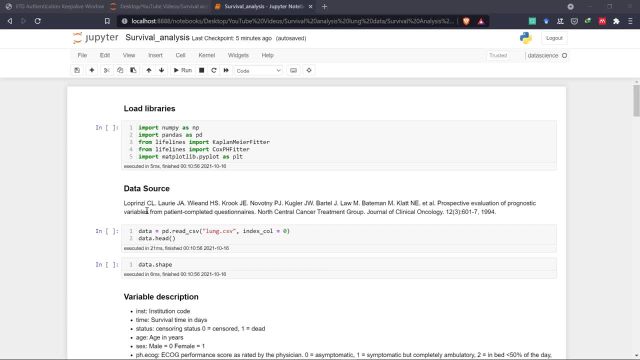 treatment group and they try to compare the effectiveness of vaccine over given duration time, like after taking the medicine or, say, vaccine if a person get affected, what is the probability that the pedestrian dry in one year, five days, ten days, thirty days? so this kind of probabilistic analysis which can be done using uh the time to event analysis. so in this tutorial we 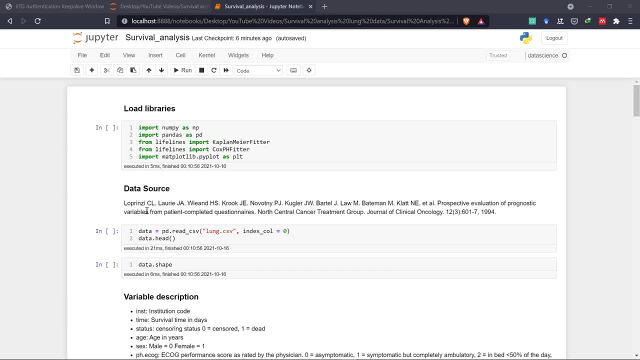 are. we will analyze the time to three types of time to vintage models. that is commonly used. one is parametric model, uh. non-parametric model, then same parametric model and parametric model in non-parametric model. we are going to use the kaplan-meier estimate in same parametric model. 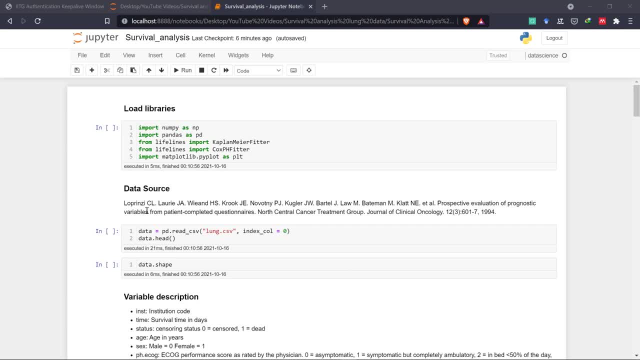 the cox is a proportional hazard model and for parametric culture model, uh depending upon other distribution such that can attribute the outcome variable. so we will let you talk about that in this video also. So for this video we are going to use the lung cancer rich data set. 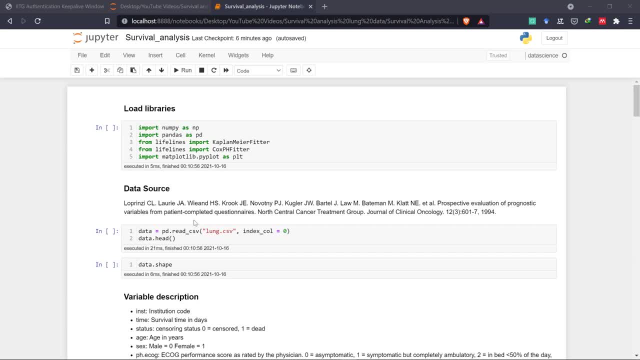 So lung csv- I have already extracted the data from this- actually comes with R, so I downloaded it from R and compiled it here, and before that we will proceed with this analysis. So first let's load the libraries. here we are going to use the numpy pandas, spd then 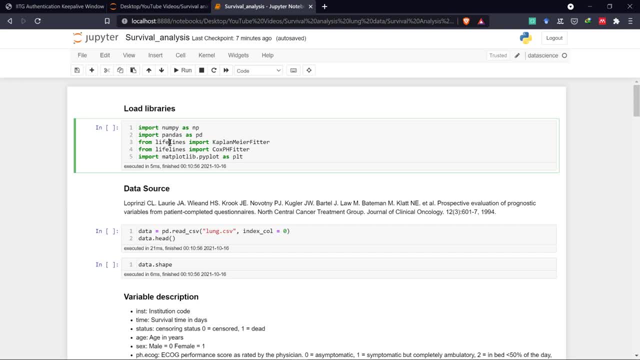 you have to install also the lifelines package for survival analysis. it is in python so you will get this either from anaconda distribution or using from the pip. you can install that, So using lifelines from that. I have imported the Kaplan Meyer fitter that will fit the. 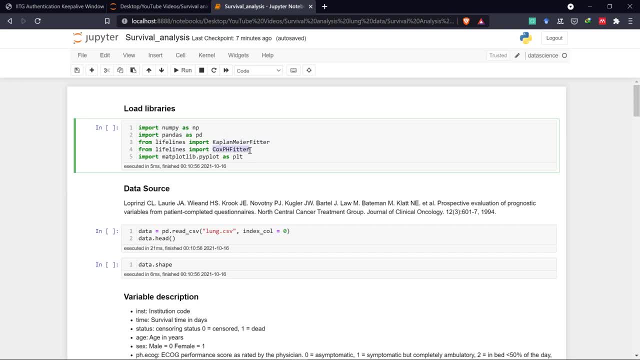 Kaplan Meyer estimator, and also the Cox proportional hazard fitter, ph fitter. Then I'm also importing the matplotlib, such a pipelot as plt, so we will plot those things. Let's first load the libraries and after that this is the data source we are going, the data 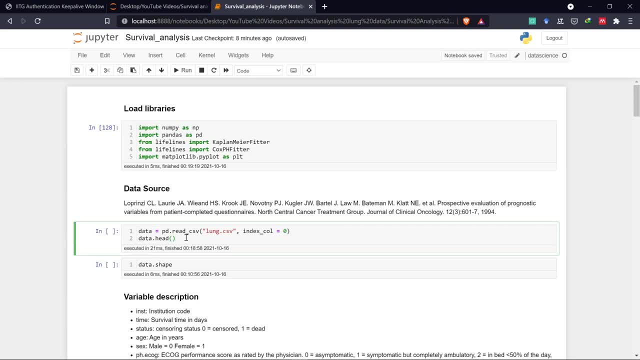 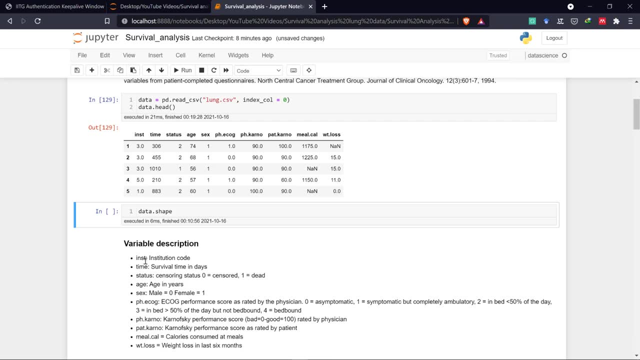 is come from this such a source, and let's load the data using read underscore, csv. and this is the data. The data consists of these such variables: first is the institute, so the institution code, from where the data is gathered. then time, that is survival time in days, so up to 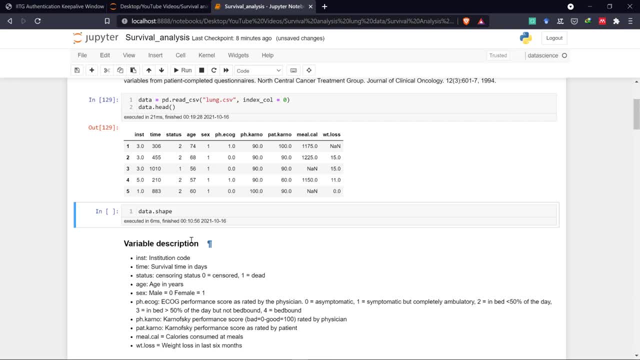 from, say, start of that observation period, up to which days they are for one year or two year, the this observation has been made. So next is status. so censored status is here. actually it is in one and two, so we will convert it into zero and one, so the data is instead the one is censored and the two is dead here. 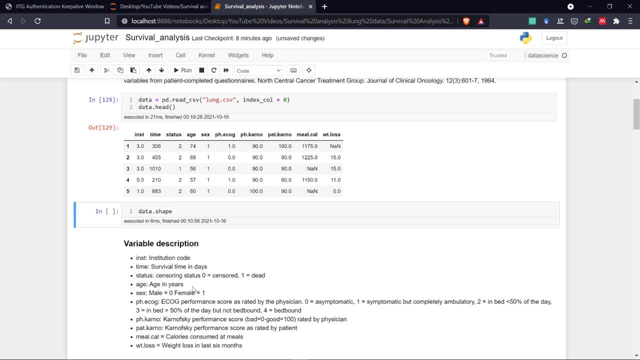 in status, but I usually prefer the base category as zero, as censored and one as such that's dead. So Here we are going to use the right censored data like this: I will convert to zero and one letter by detecting minus one, directing one from this status, so the status is censored. 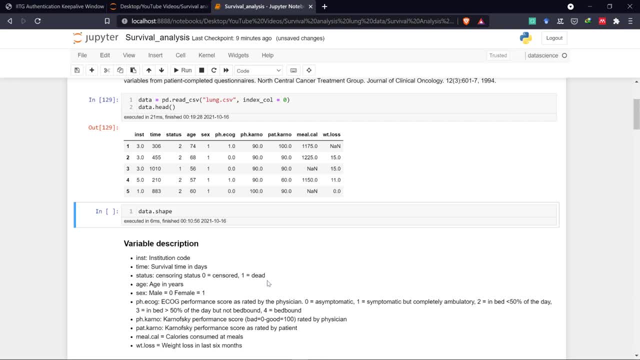 as here, zero and one is dead here, so one is the event that, whether the person date, so censored means in survival and assist. the censoring is also different types- left censored, interval censored and right censored- are there in this data. We are going to use the 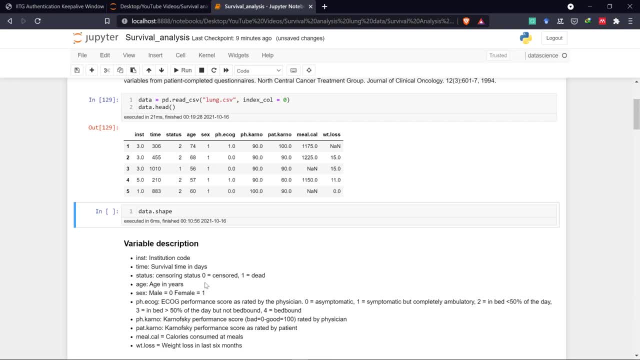 right sensor data. right sensor means here after observation, start of the observation. maybe the person dropped out from that experimentation, or but somehow the participant moved out from that experimentation, or maybe the person survived up to the extent of the observation period and we don't know what happened to that participant age: here age is in years. sex as a male is: 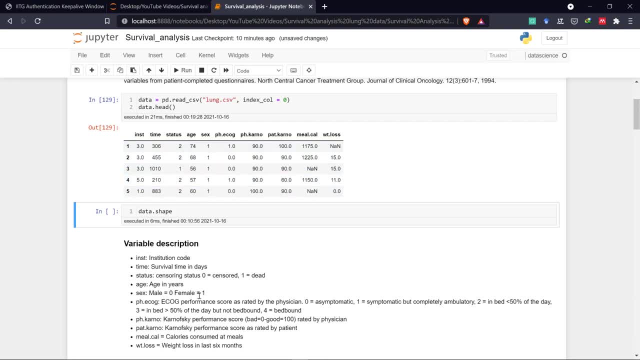 one, and female is too, but I want the male, geo, and we will one, so we will deduct one from that litter. and pH echoc is the equal performance, such as for, as rated by the physicians, zero has robotic ones, symtotic but completely ambulatory to in bed, less than fifty percent of the day. three in bed, it's a more than fifty. 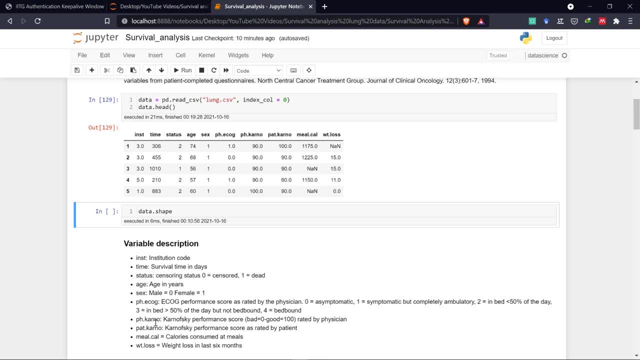 percent of the day but not build bound for bid bond and pH. Quran Karena is a Carlos Carnav sky. her performance. cool is in Judo is bad one, good is one, a rated by physician and Pat Karno is the purpose score given by the patient meal. 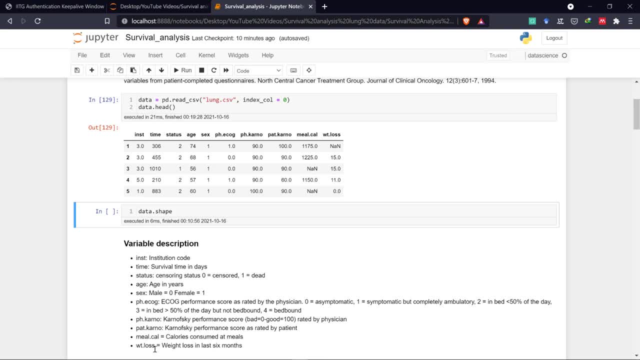 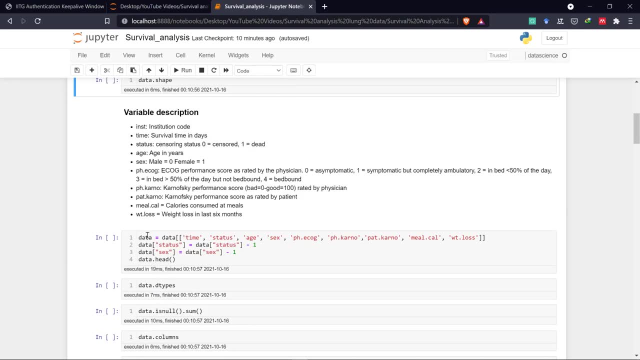 calorie, calories consumed at meals- and weight loss is the weight loss in last six months. these are the variables, and so let's first just select the all the data or columns that we are going to use and saving in the data. then, as I want, the reference category for the status that is censored or how to date that is. 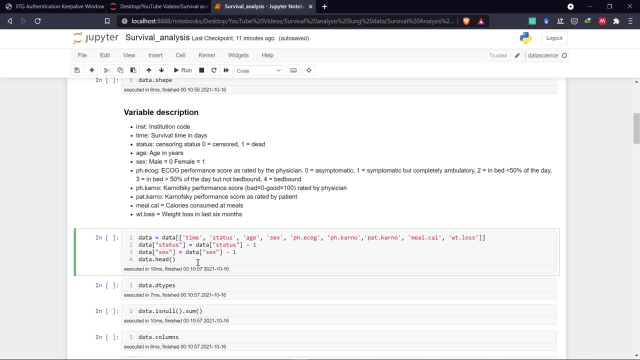 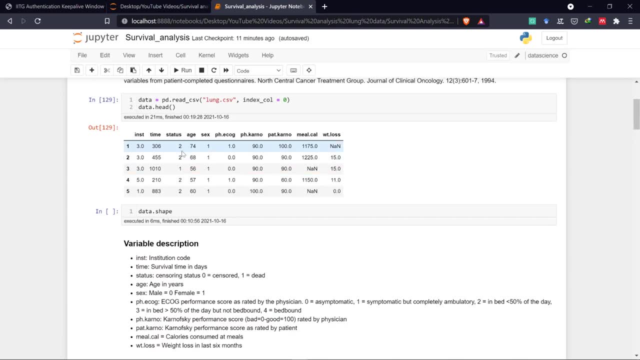 in one and two actually, but who I want? I usually prefer the base category as zero, and so we will deduct as a one from the data status. so it will make the two one and one make the one zero, and similarly I also converted the zero male and one. 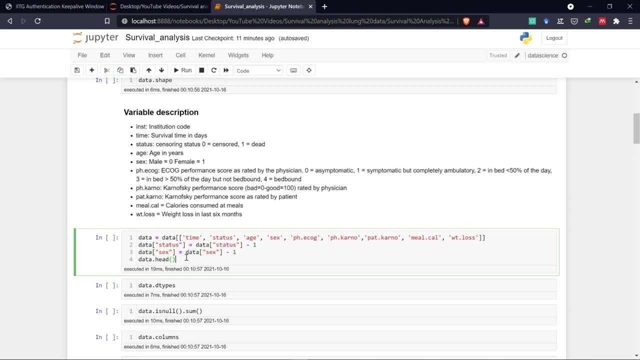 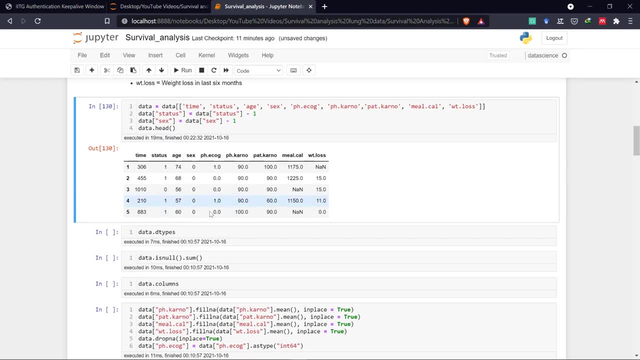 female by deducting minus one and let's check with the head and now you can see it is zero and one one somewhere I will be in later in the data middle of the rows or somewhere else- but and status is also now one and zero next to the list. let's check the. 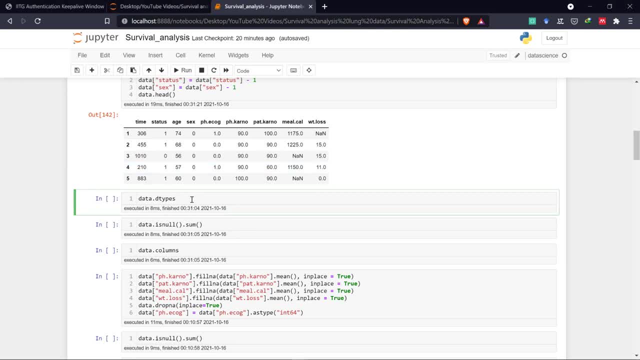 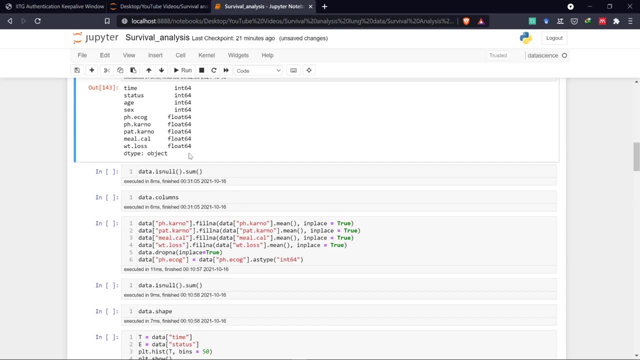 data types. so data dot, J, D types and you can see the four variables are in integer 64 and a rest of in float 64 and we also need to check whether the columns such a contain and missing values. so data dot is none function. dot H is sum method. it will give the column wise. 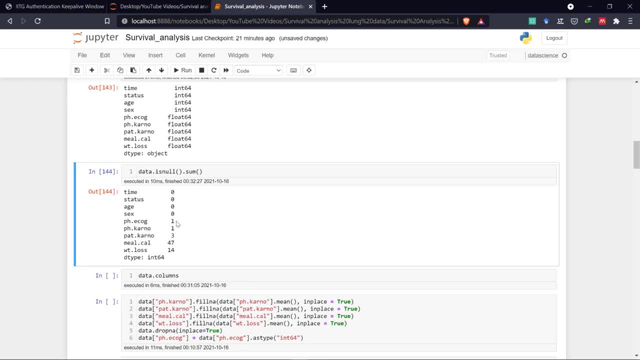 count for the missing values, the pH. yoocog has one missing value, pH, which O'Connell has one and Pat corno has three missing values: meal dot calorie has 47 and its weight loss has 14. so the this, the following columns: and where the pH. 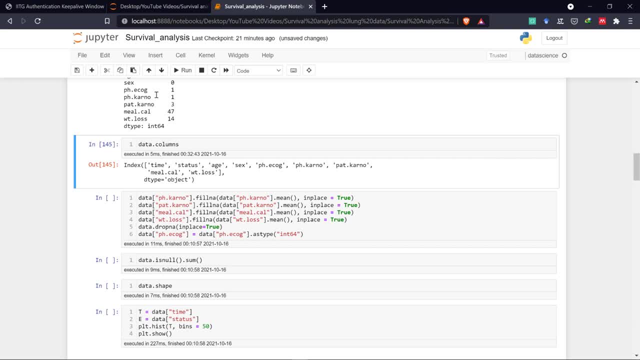 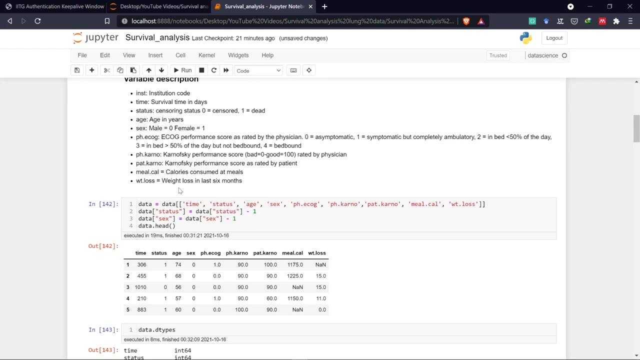 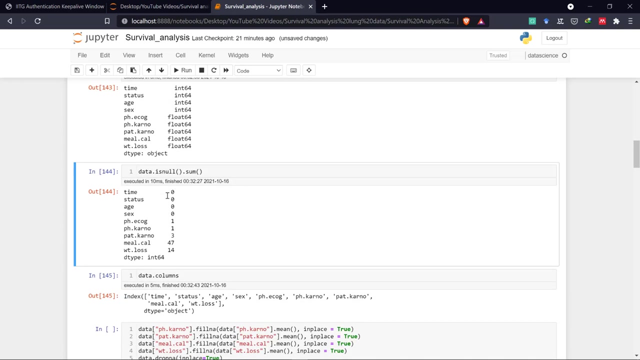 curr and the pH eco is a categorical data so we can't change it or play or say impute it with a mean value. so we will later remove it. this one observation and the total observation we have currently is around- i missed that- i guess 228 and so except ph, ecog, that is categorical, we i will replace: 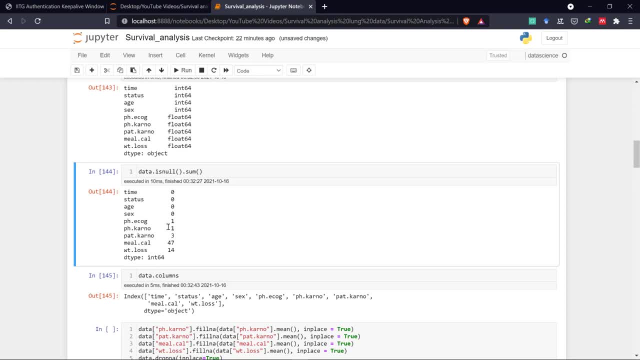 all the missing values in all other data that are continuous data with their average value, because i don't want to delete them, it is just for the demonstration purpose. if you wish, you can delete, but we already have been, we already having a very small sample, so i will replace. 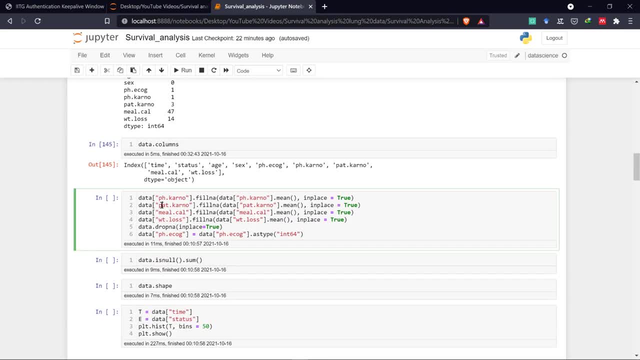 with the mean values. so here, uh, the data, the ph carno, uh uh, the column. i am using the dot filene. i am replacing with the mean and in place is equal to true for all this x, this, four variables like ph carno, pet carno, then meal, calorie and weight loss, and after that i'm 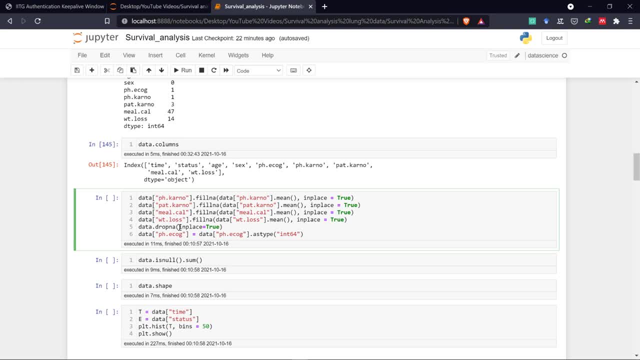 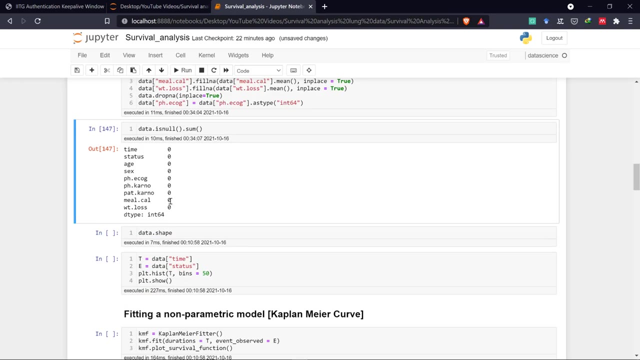 uh, removing the remaining rows with any values, that is, for ph ecog this one, and after that i'm changing the ph ecog to a integer 64 values. okay, so after that, if you again list the ns sum of the ns okay account, so here we will say that now there is no any values, or 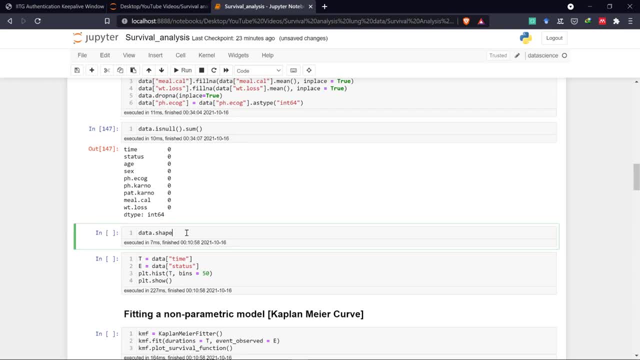 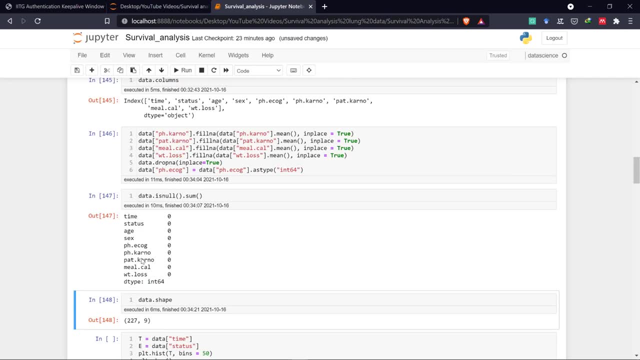 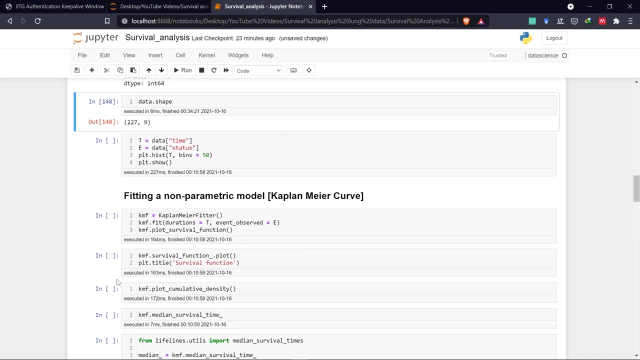 missing values in the observations. okay, and next we can check the shape. now we have 227 because we deleted one uh actually observation, that is for ph ecog. this one observation, it is a categorical. and now, uh, before we proceed with the different modeling approach, first let's just save the time observation or time column in hd and the data column, your status, in e. 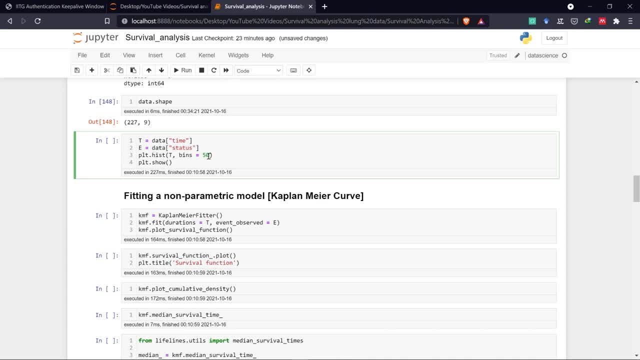 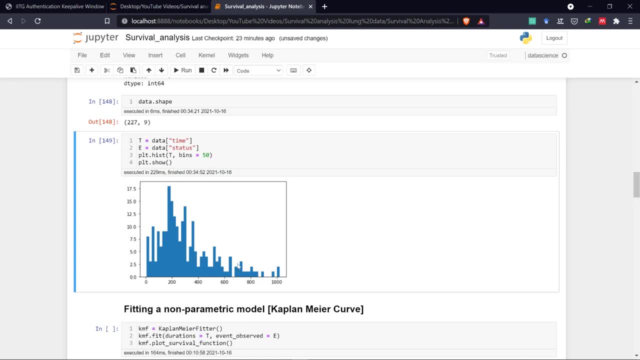 and let's plot the distribution of the time, uh, with a pdt with 50 bins using the plthist function and show this. we can see this. it is almost look like a log normal, or say we can say it is a weibull distribution, though the distribution can varies with just tweaking the parameter. it will. 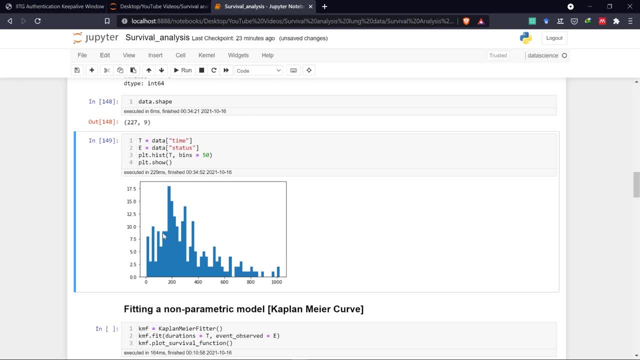 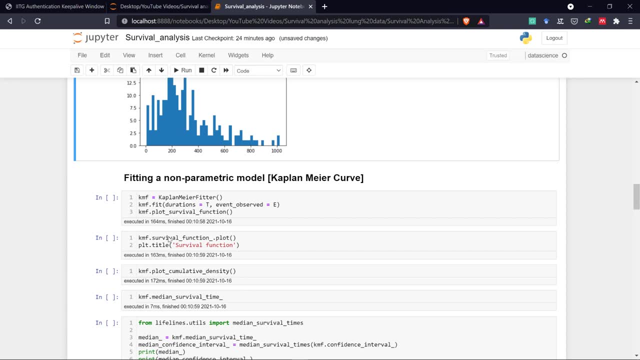 take this shape. so later we will compare in the apt model how it will look like section or which model or which distribution it really fits. so first we'll go and plot it and on the fit, a non-parametric model, that is Kaplan-Weier fitter, using Kaplan-Weier fitter, a Kaplan-Weier. 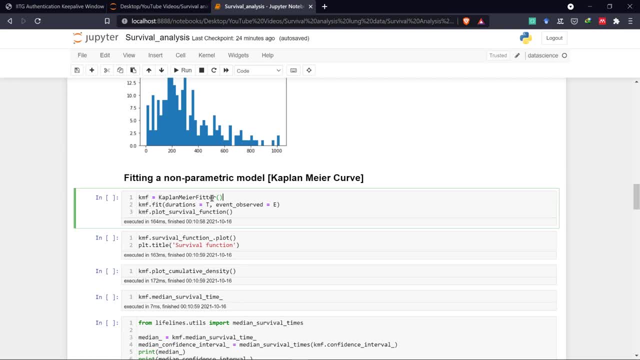 curve. so at first we will call the Kaplan-Weier fitter as a class and create object and save in kmf. so after that kmffit we supply the duration time, that is t, and event observed, that is e. we already saved the data here, and then with plot, with the kmf object, we will plot survival function. 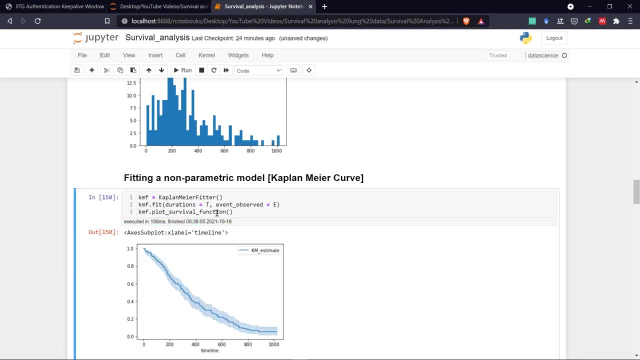 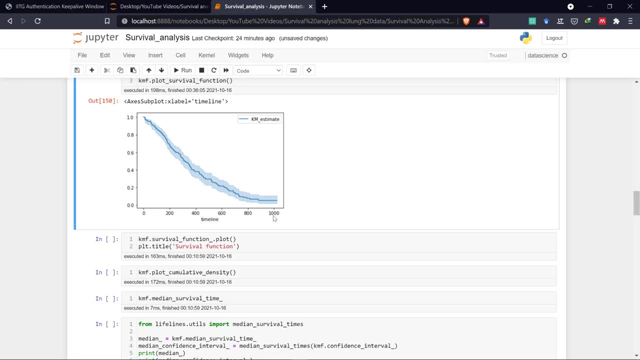 uh, this function we will call that will plot the survival function. so this Kaplan-Weier estimated plot look like this: then y-axis is the probability of survival and then x-axis such that time frame or the time duration. so, uh, for example, uh, what is the probability that a person 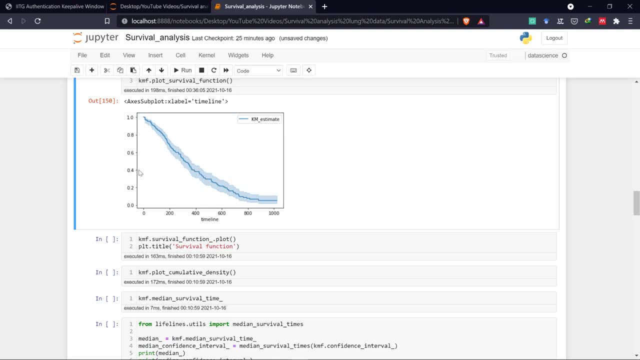 lives up to 400 days, so corresponding that that is around 40 percent. okay, so what is the 50 per? what is? what is the 50 percent survival probability? uh, or how many days 50 percent of this this observation just survives, say around? it is such a 300, uh, 80 or 310 or something like that it would. 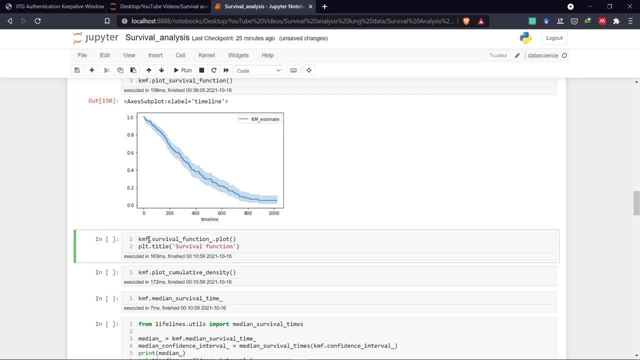 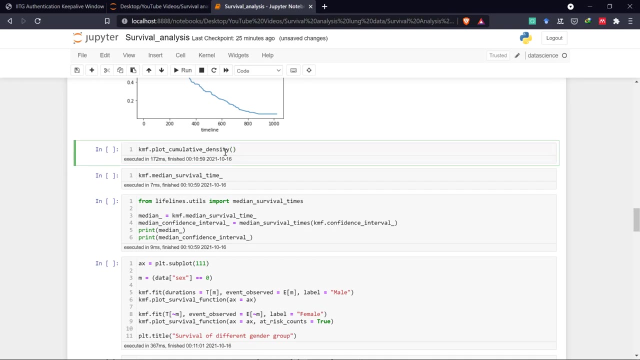 be. so we can also plot this using kmfsurvival function, dot underscore, dot plot, and that will plot without any confidence interval. and we can also use our plot, either plot as a cumulative, which of density, and it will has a plot accumulative density function. so 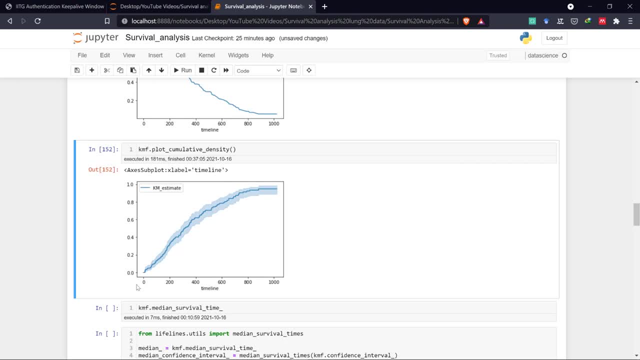 uh, it is like one minus such a survival actually, uh. so now it will show that what is the probability, uh, probability of which uh say uh, death, like uh in say 300, uh or 600, say 600 days, uh, 80 people will die, corresponding approximately, if we just uh. 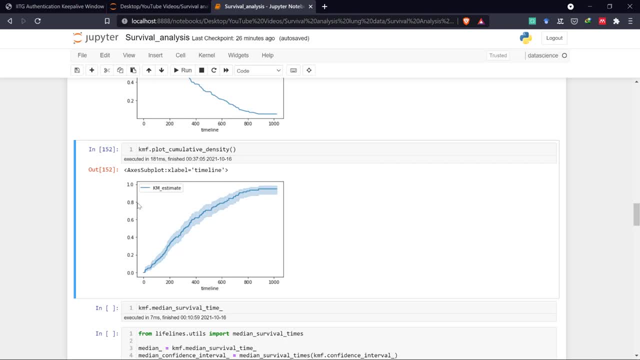 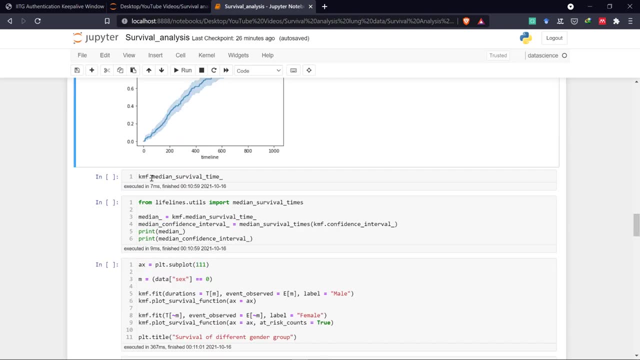 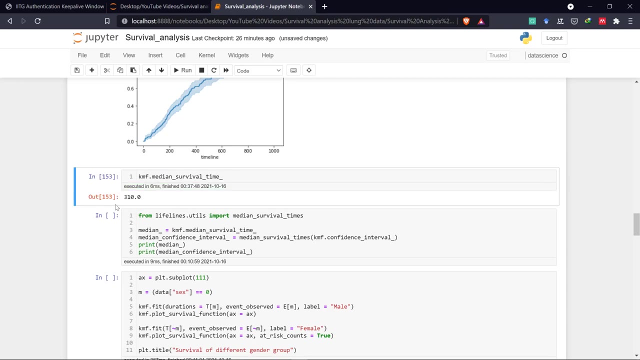 uh draw a line corresponding 600, that 80 percent of people will legit die or not survive. it's opposite of that. so we can also estimate the median survival time by calling the dot median survival time. that will give the 50 percentage of survival, 50 probability of survival, uh that 310 days such 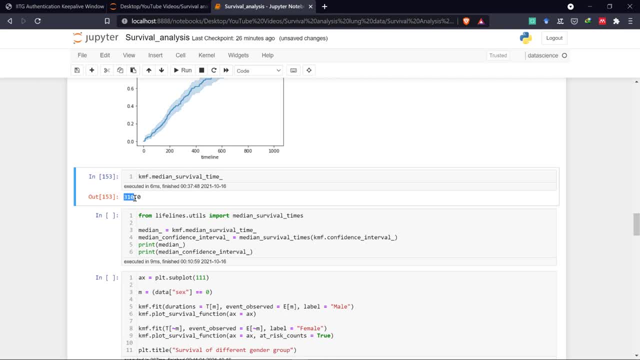 a 50 percent of the observation will survive and 50 percent will die. that is the case. so we can also use uh the uh from lifelines such a utility. so we can also use uh the uh from lifelines such a utility. so we can also use uh the uh from lifelines such a utility. how we will import the median survival. 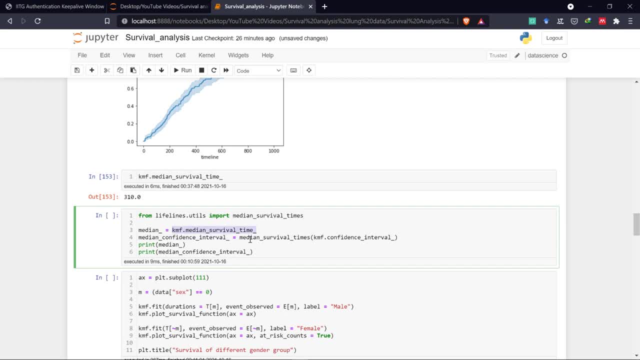 how we will import the median survival times. we can compute the kmfmedian survival time and also compute the medians uh. use this such a median survival time search function and supply the kmf confidence interval. that will save in median confidence interval and we can print both of this. 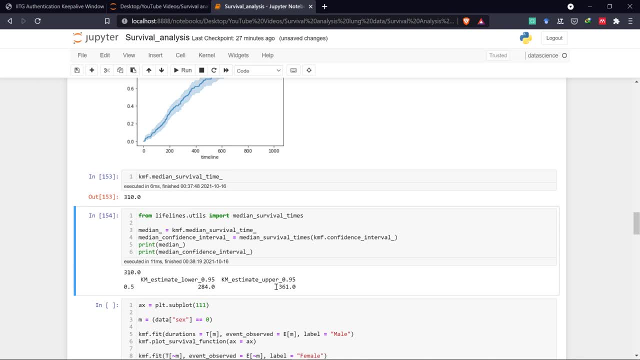 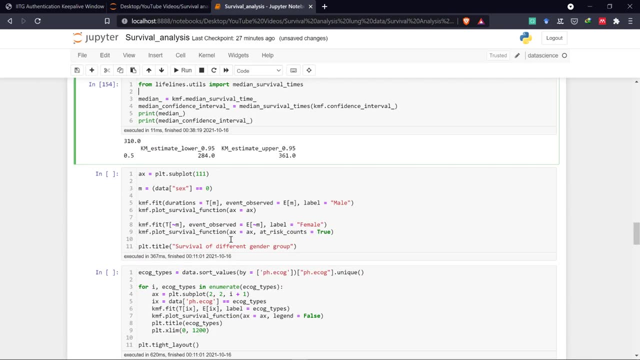 so the median survival is 310 and the confidence intervals are 284 to uh 3861. okay, so 95 percent confidence intervals are there. next is that in kaplan meyer, uh, kaplan meyer curve, uh, we can't use such um. uh, we plot, we can plot the survival function, but we can't just. 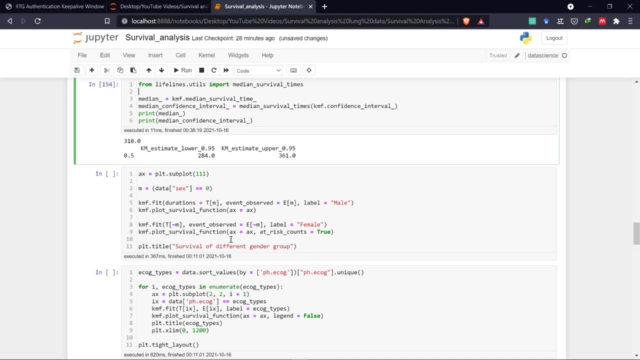 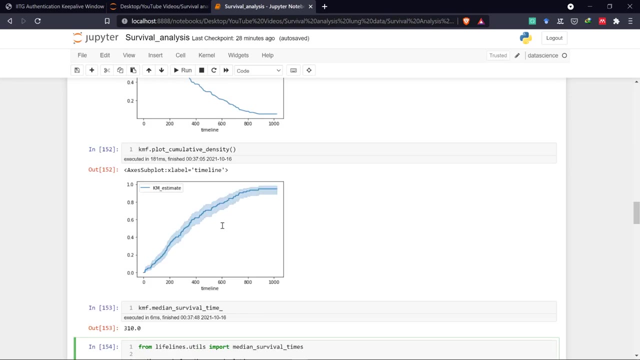 observe the impact of the different predictors. we can use such a few categorical data and, based on the subset of data, we can plot different survival curves and compare them. and it has also some limitations. like it gives, the step functions like uh, the function is not smooth and if you have a 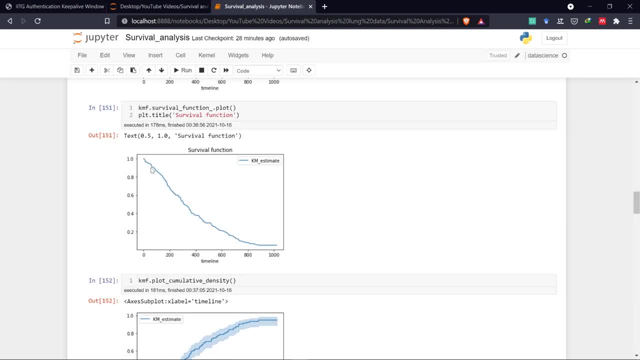 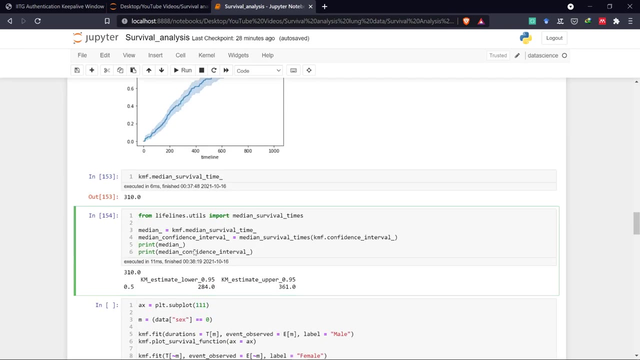 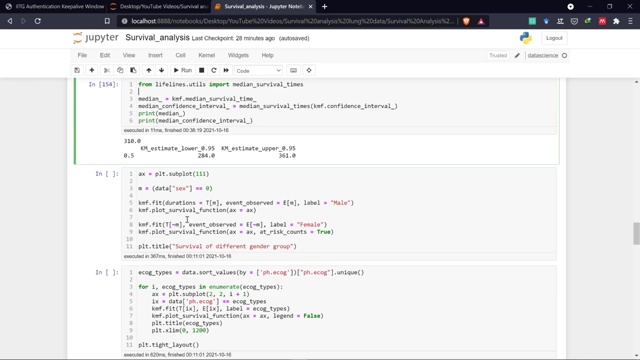 bit limited to the sample, then this such a function will, uh, give some say over a given over if the probability remains such a constant over a given duration of time, which is not also practical or realistic. so in this case, if you want to compare some different groups, we can also do that in using this by segregating or by 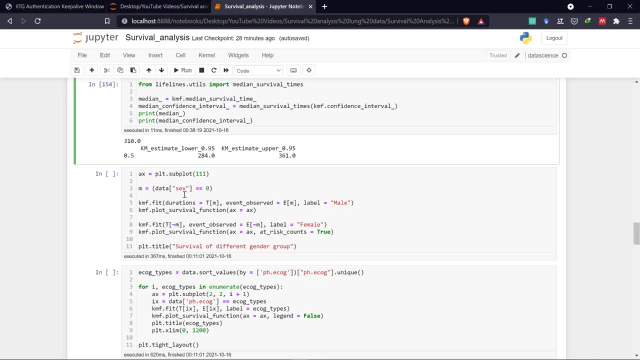 using the sub subset of sample of the data based on a particular group. for example, if we want to plot the difference, uh compare the survival curves for a gender group, like for male and as a female uh patients separately, then first we uh here uh. i have also given this code, so in ax i am uh supplying the plt subplots. 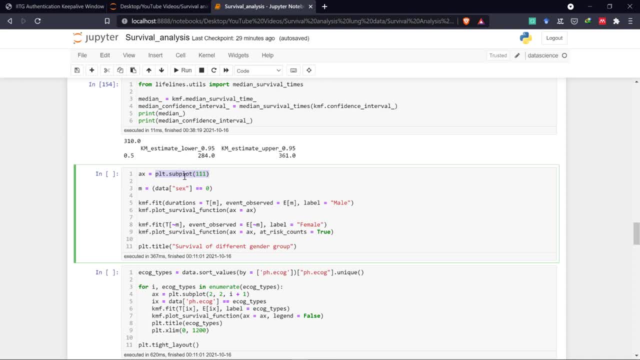 one, one, one that is a in single plot we want to uh generate, we want to impose the male and female, such as survival, such functions. so i'm using the creating a mask for where data sex equal to zero, that is, male, and saving in m, and also kmffit duration is equal to t. from that i am. 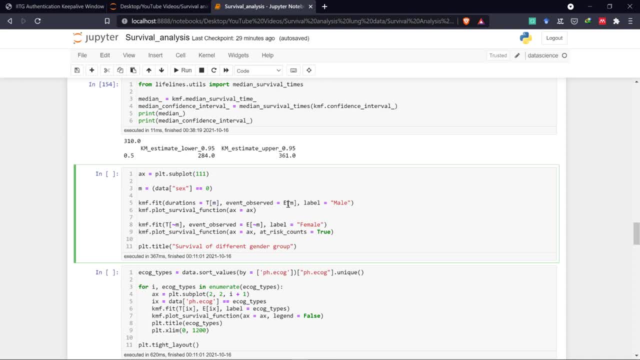 subsetting the male where the due to male is true and also the male observation, so the time event observations are true, and labeling that male and plotting the function in axis, ax similarly for a female. i'm while indexing, i'm giving a tilde sign, so it will. 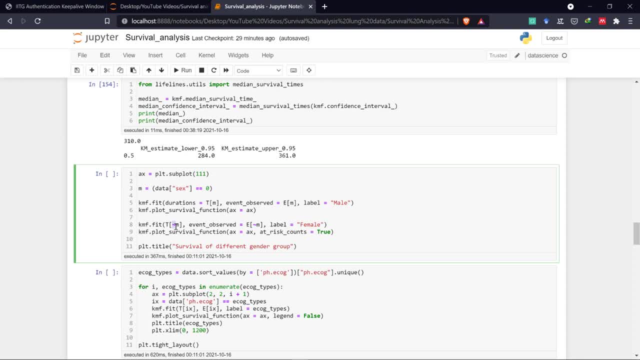 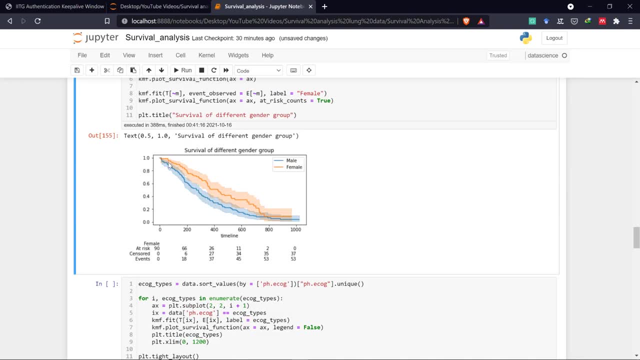 exclude where it is true, that is male is true, and it will select only the female, and i'm plotting and limiting. this is a female. if you plot this, this will plot two separate curves. the orange one is for female and the blue one is per male, and you can see the female have more. 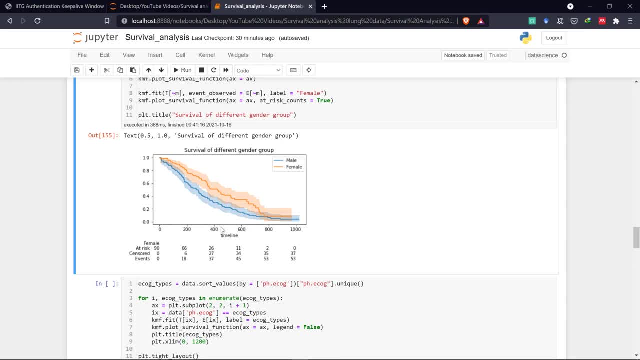 survival of probability at given at a given instance of time. if you check, the female has more survival probability compared to its male and this is also i'm also giving the at risk. true, give a risk at risk table in tabular form. so how many patients are at risk? 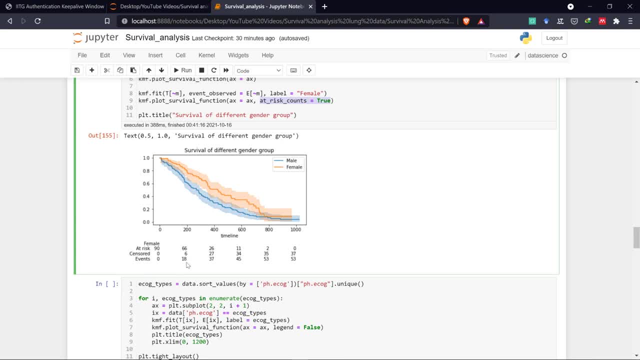 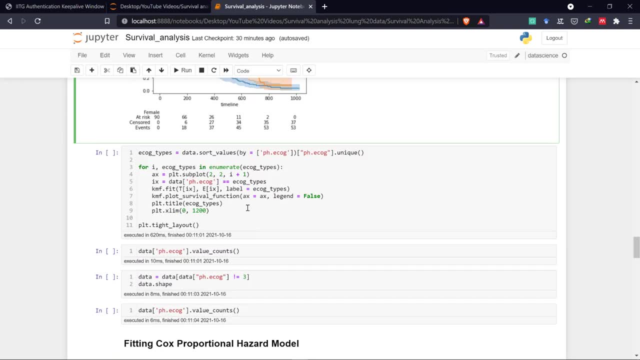 how many are censored? what, how many of events happen? events were occurred. it will also tell. is that over a given how? about the given duration of time? next, we are to automate the process. we can use a for loop, and if number of categories are more, then you can use a for loop. so here, from data I am using, 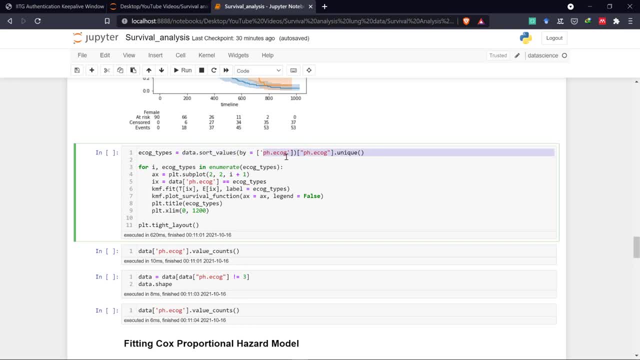 the sort values and shorting th equal from 0 to same up to 3 and selecting the pH echo can identify the unique values. then I am using a for loop. I is the index and eco types is the values in enumerate eco types. this unique values. 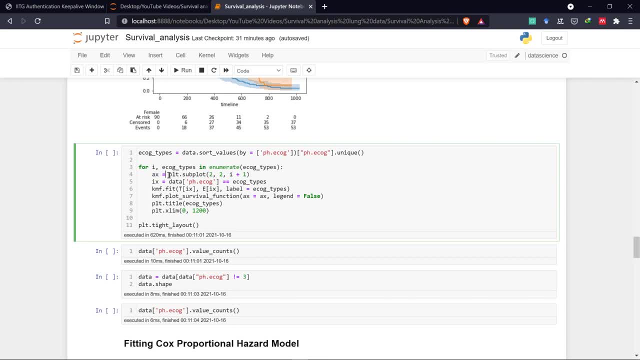 then I'm supplying a axis, creating axis object. we have to do surplus 2 by 2, that is such a 4 plots 0, 1, 2, 3. so and increasing the counter by counter value, by increasing the counter value, by increasing the counter value by: 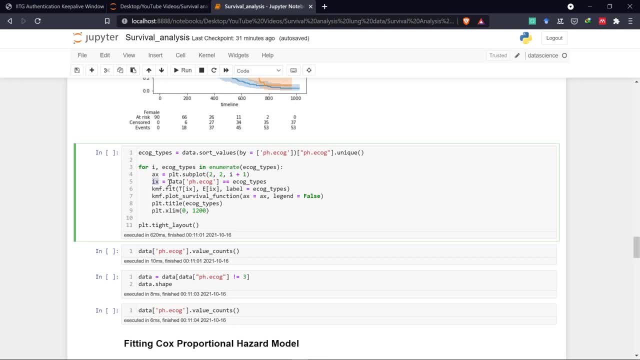 plus 1, and then I'm defining the act IX where the supplying the data PS dot, ECOG, equal to equal to ECOG type, like say, first one is 0, then second iteration 1, 2, 3, like this, and then I am fitting the model and plotting the cyber plots in. 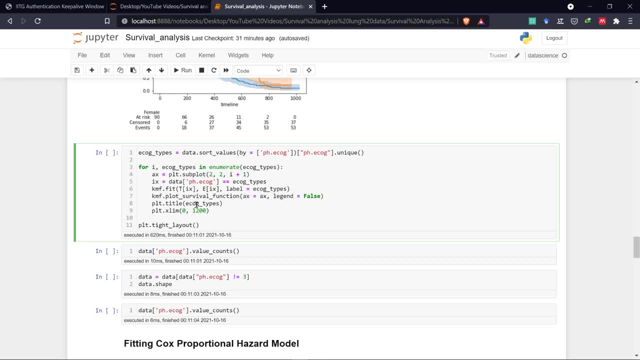 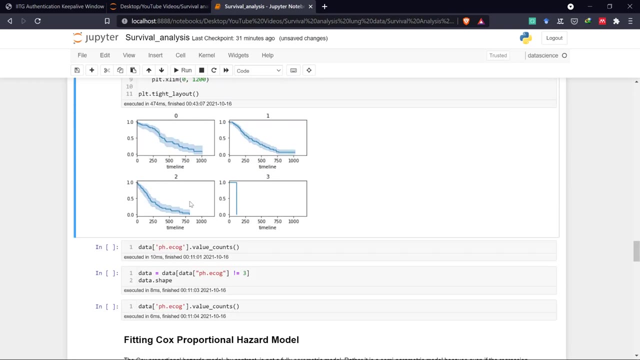 that axis and legend is false. the title is the ECOG types. based on the ECOG type it will title and the X limit is 0 to 1200. so PLT dot tight layout. it will compact the plot and if you plot this, it will plot for 0, 1, 2 & 3 for 3. you can. 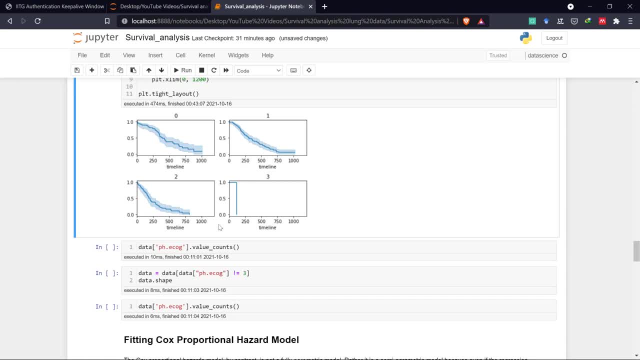 see that the plot is not good because I think the observation is- you know it doesn't have actually much a large number of our samples or observation. we can check using the data dot, pH, ECOG, dot, edge value counts and you can see the third level have only one observation. we can drop this observation. so I'm 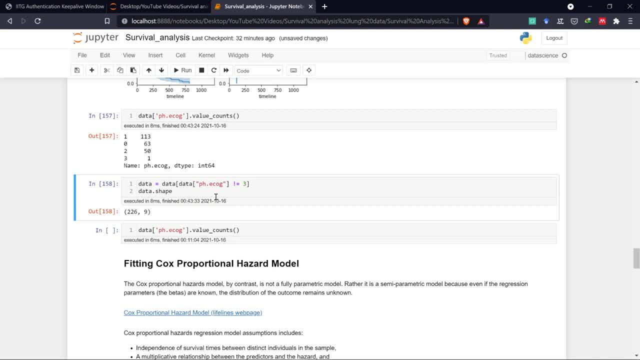 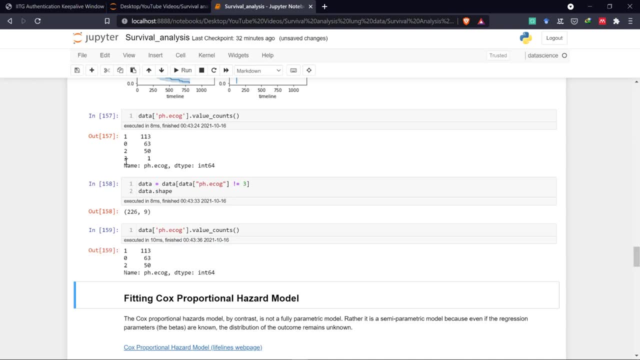 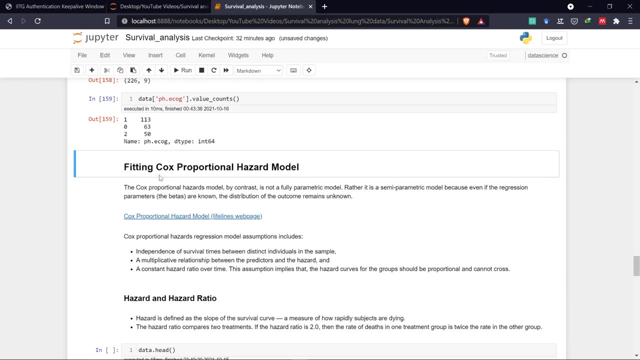 dropping it here and again. if we check, we have now 0, 1, 2. okay, so 3. we have dropped the three category because it has only one observation. now let us go for the next version of the model that is known as Cox- proportional hazard model. so Cox. 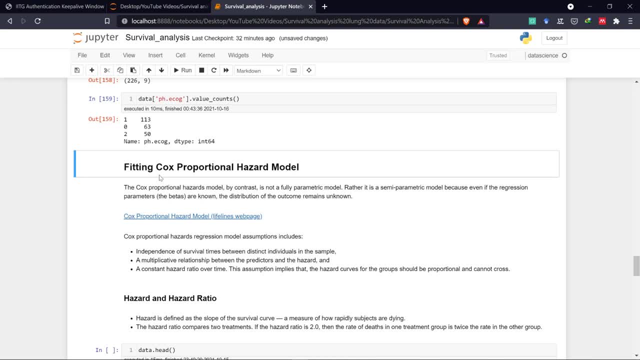 proportion hazard model is a semi parametric type of model, say parametric, which means that Rather it is semivariate model, because even if the regression parameters we can obtain the regression parameters like betas for different predictors, still the distribution of the outcome variables is unknown, like the distribution of the outcome variable is not known here. 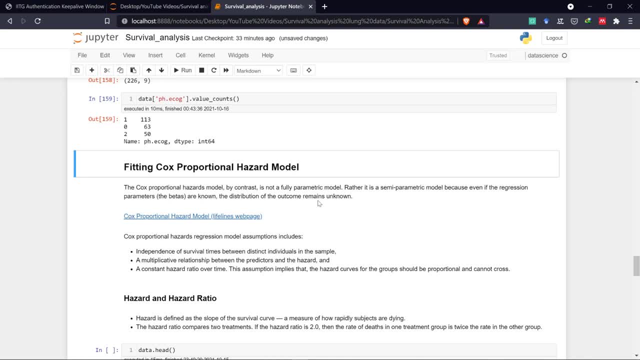 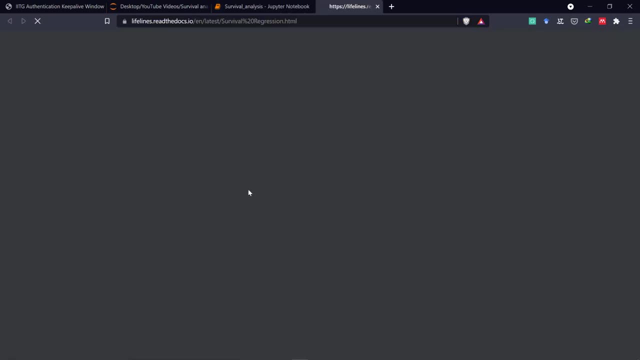 Only for AFT model. we can get the. initially we will get the. what kind of distribution the outcome variable follows the here we will don't know, actually, even though we can identify the impact of different predictors in time to event analysis. So if we can go this to this page and we can a little bit read about the Cox proportional, 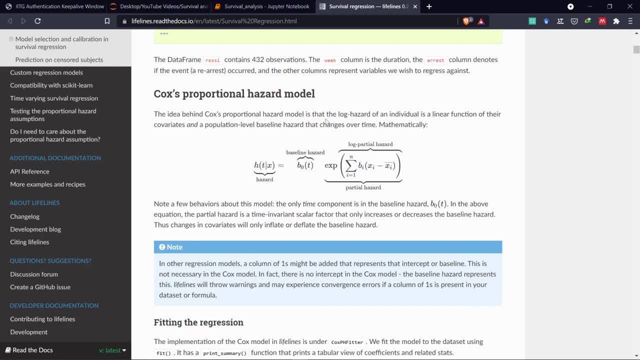 hazard model. the idea behind Cox proportional hazard model is that the log hazard, or what is hazard, I will discuss after that. So the proportional hazard model is that the log hazard of an individual is a linear function of their covariates and a population level as a base hazard. 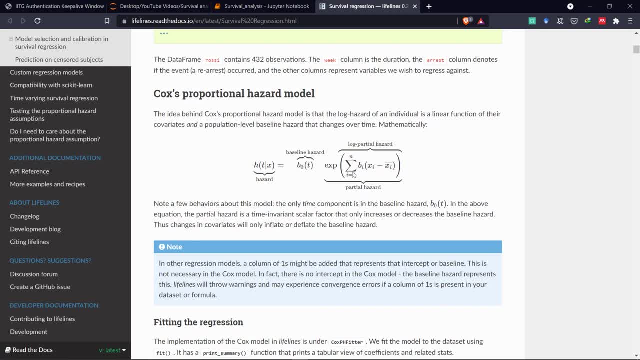 So this is the base hazard and this is the linear function Of their covariates, individuals. So this is the product of that which will give us the hazard. actually Note a few behavior about the model. the only time component is in the baseline hazard BT. 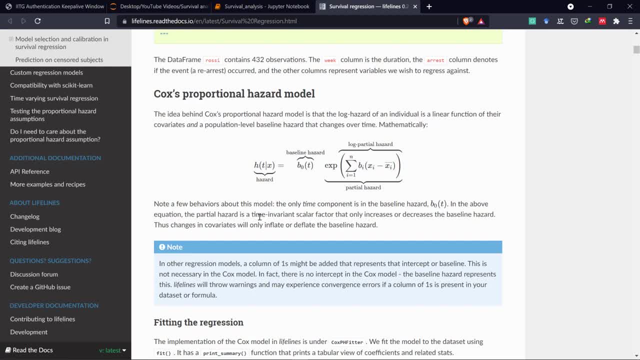 it is a baseline hazard in the above which equation the partial hazard is a time invariant is a scalar factor that only increases or decreases the baseline hazard. So, based on the covariates, it will just changes, such the baseline hazard. baseline hazard goes up or down. 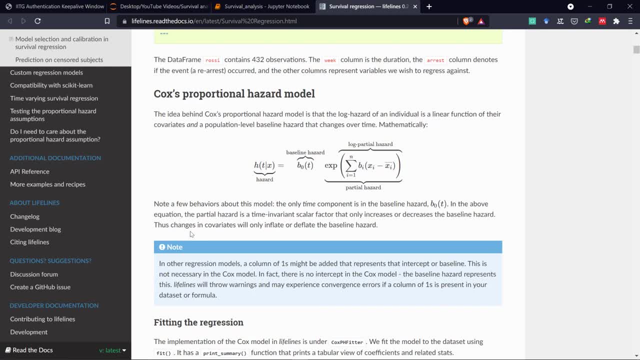 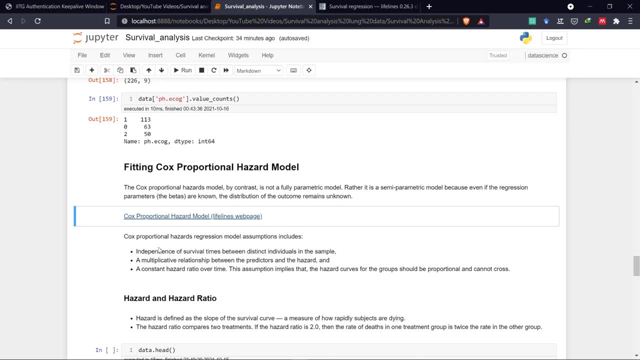 Okay, The changes it covered. so the changes in covariates will only inflate or deflate the baseline hazard. So let's go and see what are the. also assumptions exist in Cox proportional hazard model. So first assumption is that independence of survival times between distinct individuals. 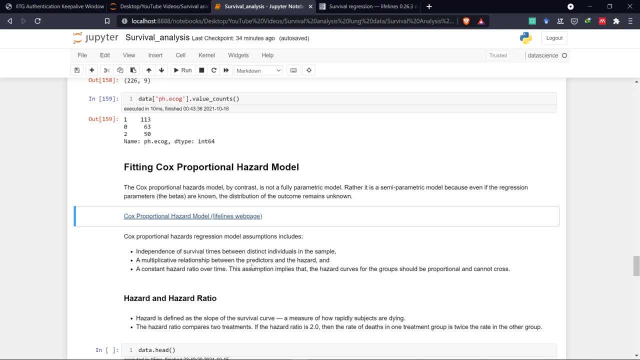 in the group in the sample, a multiplicative relationship between the predictor and the hazard. So this is the multiplicative And multiplicative Multiplicated effect and a constant hazard ratio over time. That means such the assumption implies that the hazard curve, such for the group, should. 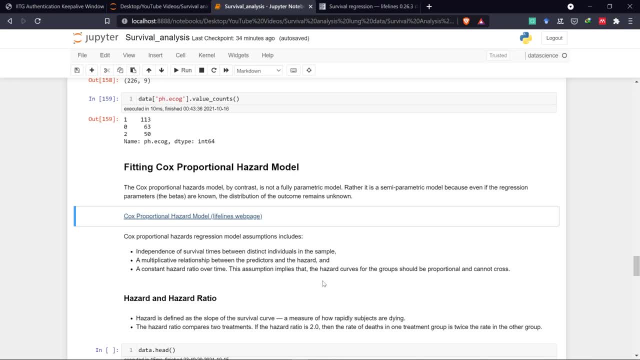 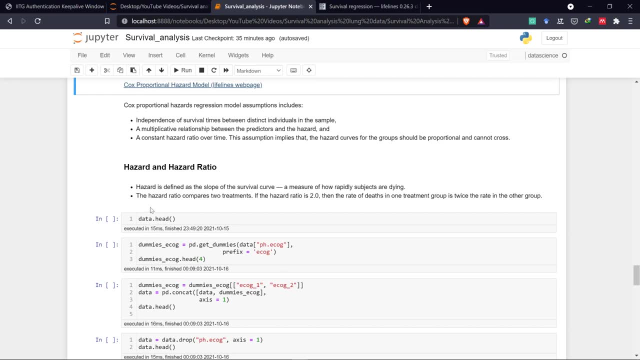 be proportional and cannot cross that assumption. we will try to see once we let's fit the model. and so what is hazard and hazard ratio? hazard is defined as the slope of the survival curve, So a measure of how rapidly the subjects are trying. Okay. 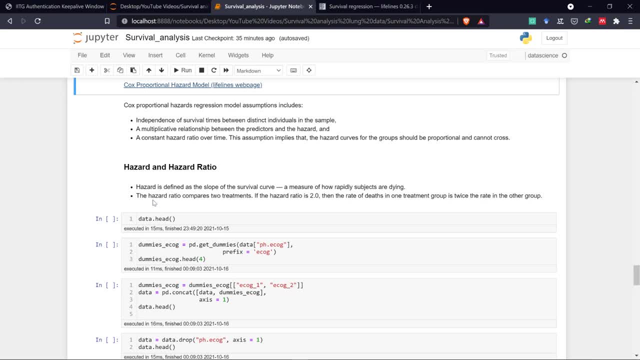 So the hazard ratio will be the comparison of two groups. Okay, So the comparison of the two groups is hazard. actually, say, if you have male and female in gender, then you can compare. what is the, let's say, if the hazard ratio, if the hazard ratio. is, for example, if the hazard ratio is two, then the rate of death is in one group, treatment group or one group is twice as that of other group, like, for example, the male having twice such hazard as a female. in many cases this happens that male has such more hazard of. 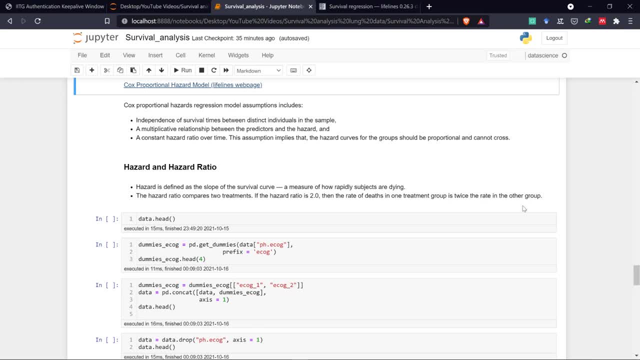 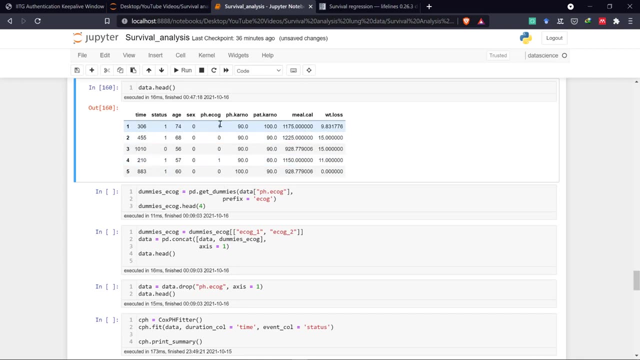 dying Due to heart attack or other cases where females have more survival chances. So let's see the data first and you know we can see that the sex and the PHE Cox are categorical. here we treat it as a categorical but for modeling purposes we have to if we 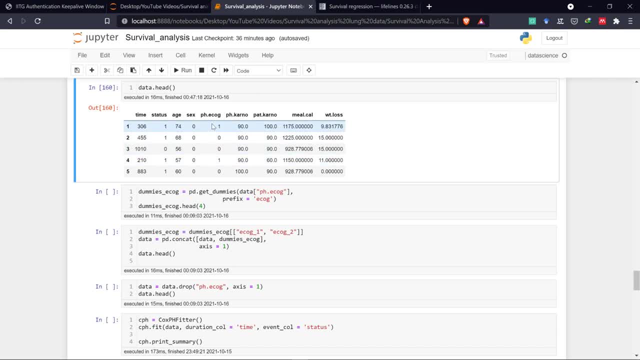 have more than two categories. we can usually dummy encode those search variables for analysis purposes. If you, if it is for publication that you have to do in first hand, before you you apply the or fit the models, and if it is for some production level or just for prediction purposes, then 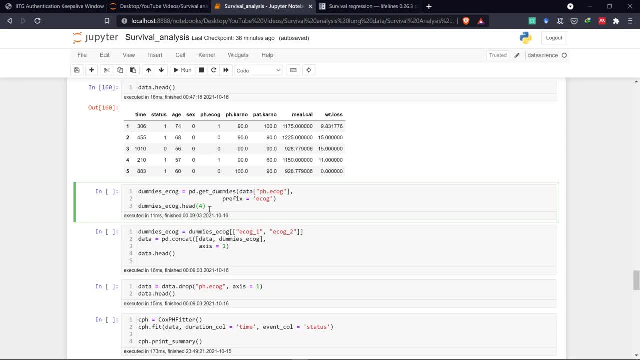 you can, as you go, with this also, but that will it improve the accuracy. So here the we can use the PD dot, get dummies and supply the PHE Cox. I'm not going to be coding the sex variable because already it is in zero and one. 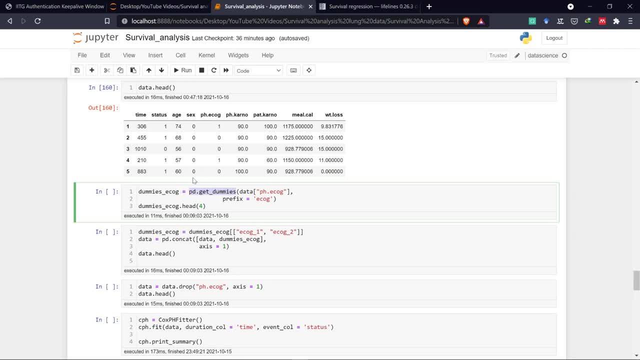 Okay, And if you want to alter like one now is zero is male, one is female- If you want to do alter like zero female and one male, then you can again dummy code and change this. But here it is OK, and zero is male, one and one is female. 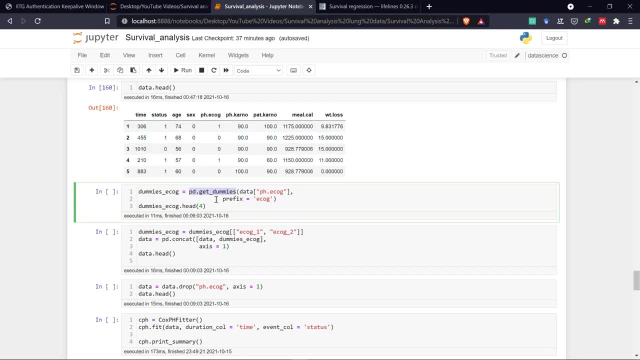 And for PHE Cox. we have zero, one, two, three categories. I guess three categories we have, yes, zero, one, two for PHE Cox, and if we use the PD dot, get dummies and supply the column, And if we fix this, he caught, and if we plot this, bring this. then he called zero equal. 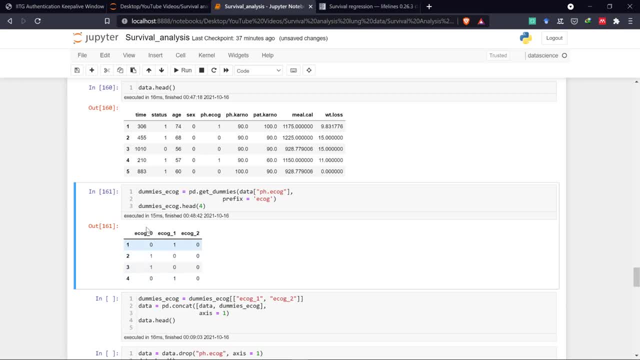 one equal two, so equal zero is the base category. we can remove that one. So how it works, like the PHE Cox is one for in one category, the first of this one, then it's zero, So in zero category it is one, then again zero. zero. category set one, then again one, so in 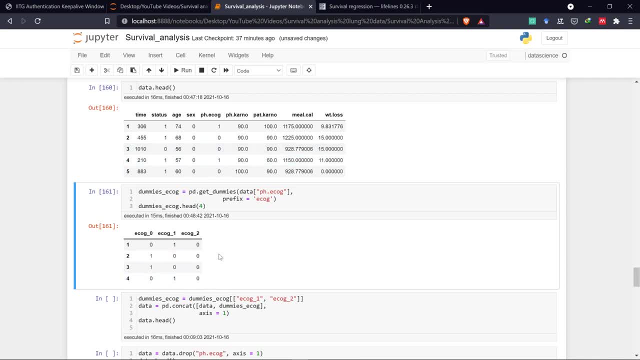 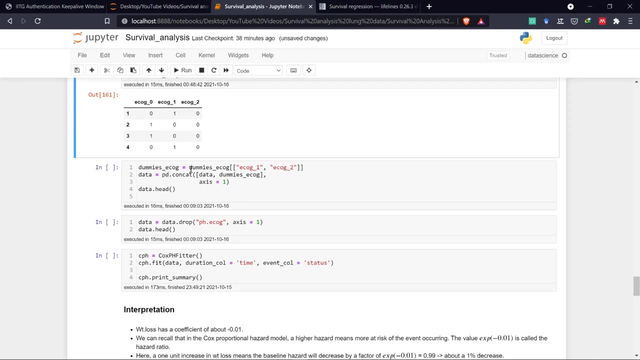 one category, one like that. if it is two, then in two category it will be one. And so For The base, for base category, we can remove this equal zero and just compare equal one and equal to OK. So next is, after the dummy coding, I'm selecting this equal one and equal two and then concatenating. 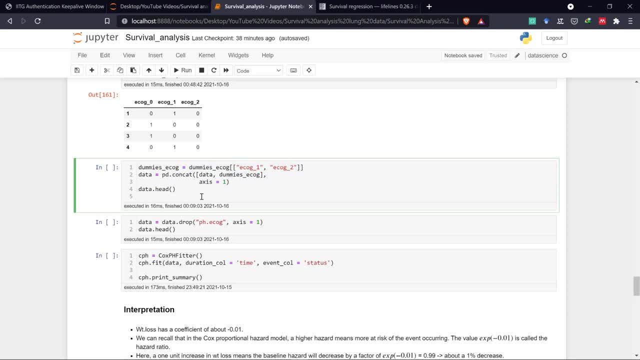 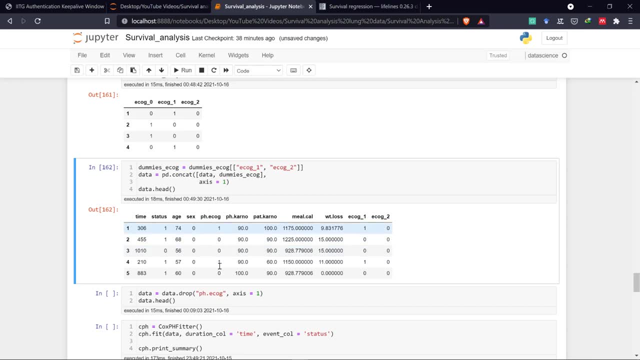 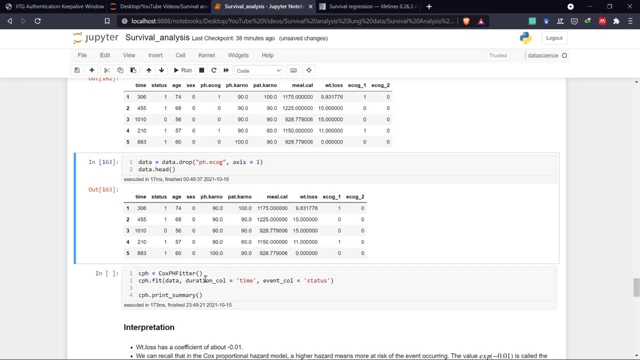 with the original data set at axis, one that is with column and in the column direction, column wise, and you can see that equal to. but we have also the PHE Cox. we have to drop that column. so I'm dropping this And now we have the final data set that we can use for Cox: proportional hazard modality. 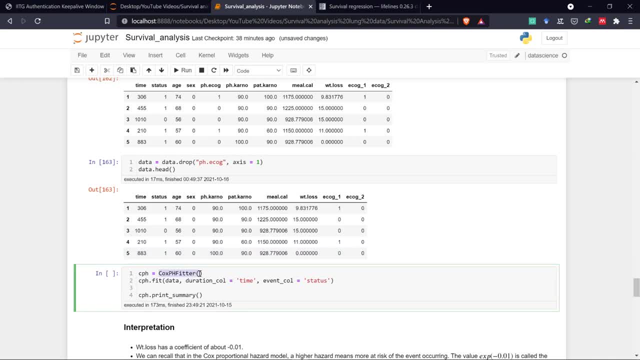 fitting. so we can call the Cox PHE class object and we'll save instantaneous. instantiate a object and save in CPH and after that it fit that we're giving the data, the new refined data and the duration: column is time, even column is status and we are also plotting. 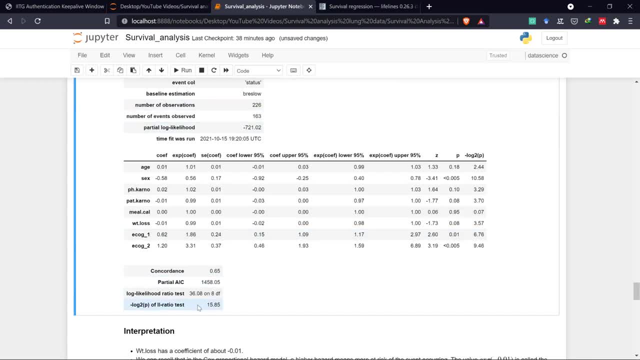 the summary. So, So, So, this is the summary. this, the coefficient, the exponentiated version of the coefficient, are known as a hazard ratio here, and the concordance index is the one of the major. it is 0 to 1, so 0.65 is I guess it is 0 to 1.. 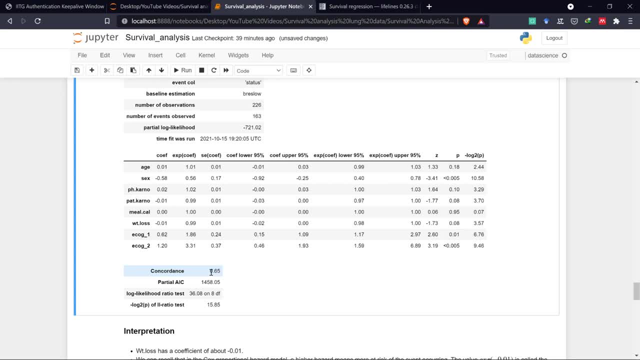 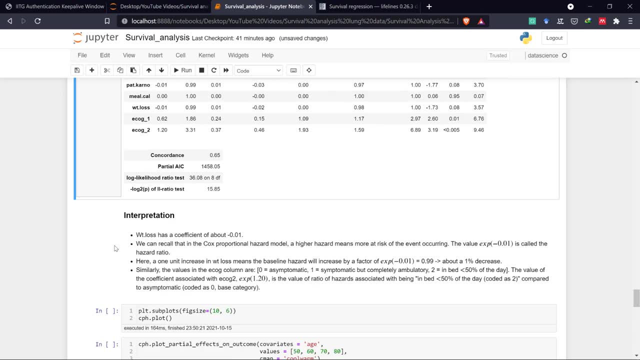 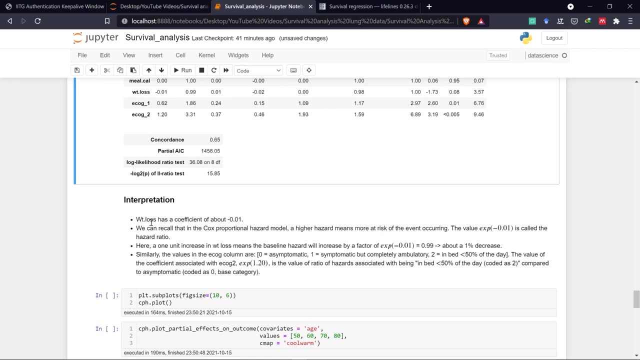 So the 0.65 is overall a good fitted model and partial AIC 1, 4, 5, 8 and log likelihood ratio test is there. So So how will it interpret this model coefficients? So the weight loss having a coefficient of minus 0.01? who we can recall that the Cox? 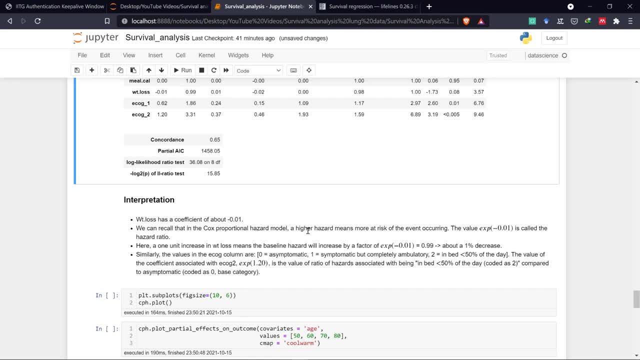 proportion hazard model. a higher hazard means a higher. that means that you're more at risk of it even talkering the value exponentiate. if we exponentiate this 0.2 minus 0.01, it called the hazard ratio here, a one unit increase in weight loss means the baseline hazard will. 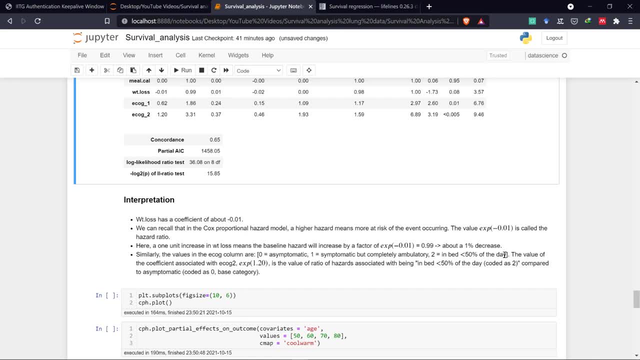 increase by a factor of 0.99.. So about one percentage decrease actually. Similarly, the value in the equal column are: 0 asymptotic: 1 asymptotic, but as a completely ambulatory to in bed, less than 50 percent of the day. the value of the coefficient associated. 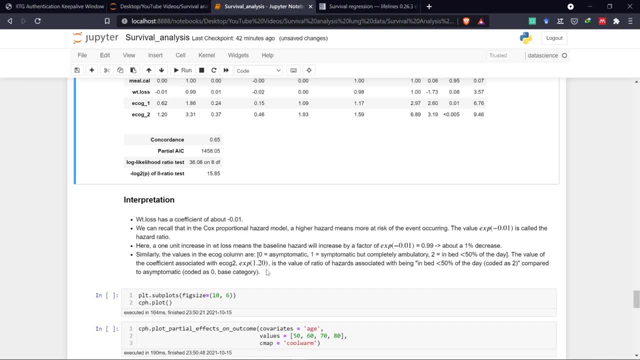 with the Cox to here is 1.2: 0.. So exponentiate version of this is 3.31. is the value of ratio of hazard as it being in bed, which is less than 50 percent of the day compared to our base category, that is, as a. 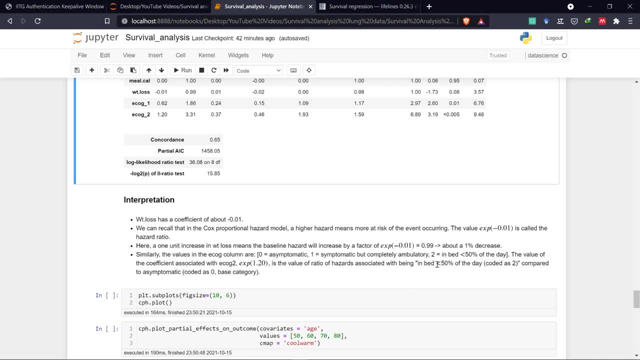 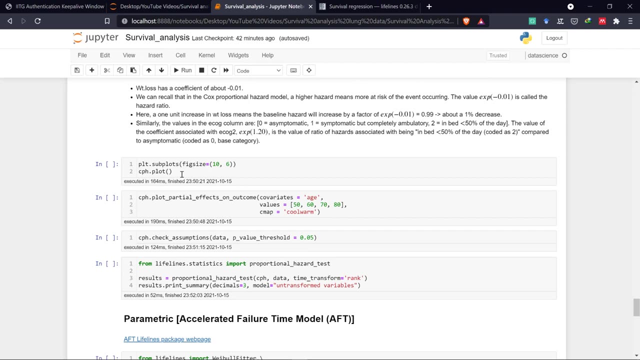 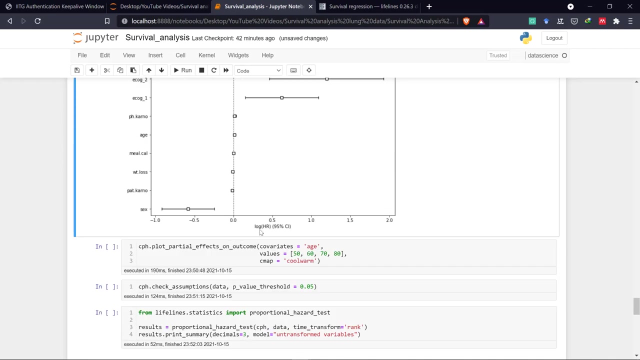 result of asymptotic. So, compared to asymptotic, those are in bed less than 50 percent of the day and their hazard ratio is 3.31.. So their chance of dying is 3.31 times actually. So next is plotting the differential coefficients in terms of log hazard. 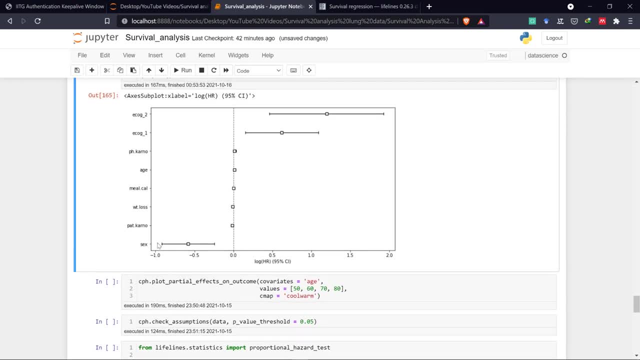 So you can also plot this And After that, if you want to say, plot the survival functions for the different covariates, for example, I want to plot the survival function for different age values. So you can use this CPH plot partial. you can use the CPH to plot partial effects on its. 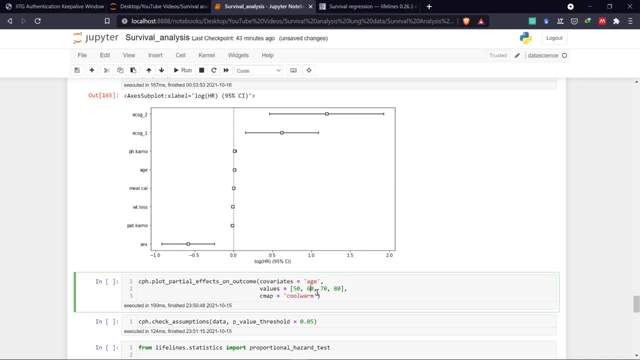 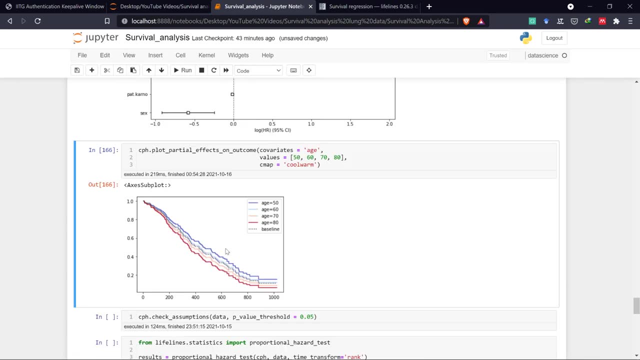 outcome then covariates is age and values are ascending: 60, 70, 50, 60, 70, 80 and C map is color mapping is cool, warm. You press control enter. It will plot The survival functions and the dotted one is baseline. sub blue ones are having higher. 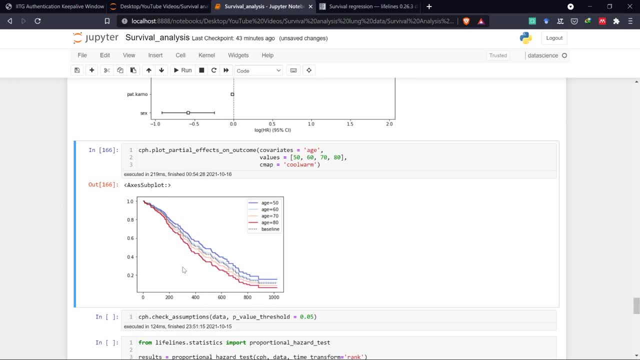 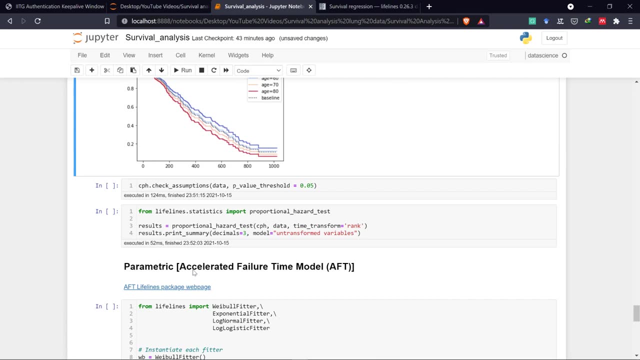 survival probabilities or through over the duration and 80 years age having lower survival priority. So older people having lower survival is probability. So next is such. we have one such. we feed the Cox proportional hazard model. We need to check the proportional hazard assumptions. 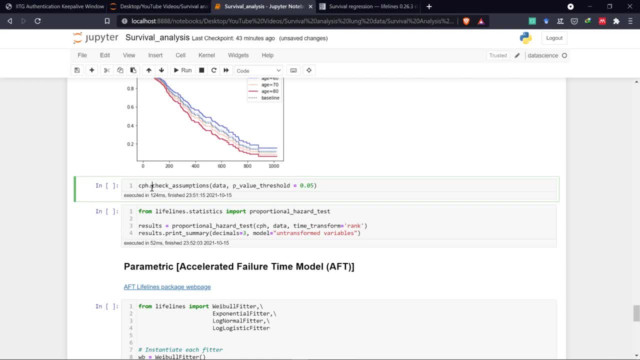 We can use check this using a log log plot. Also we can use the Kaplan Weier estimate, Kaplan Weier curves, but for a large number of categories it is very difficult to observe. It clatters the plot. So for we can use the lifelines package includes different terms of mechanism. 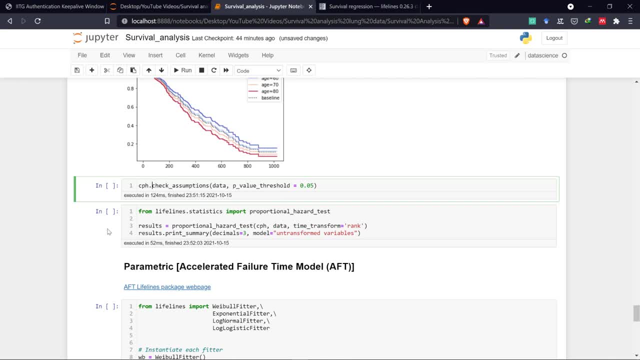 You can read about. that is in lifelines such packages. documentation here in it includes: we can do that using CPH dot. that is our fitted object dot check assumption. Assume Check assumptions And data: eddp values of potential is 0.05.. 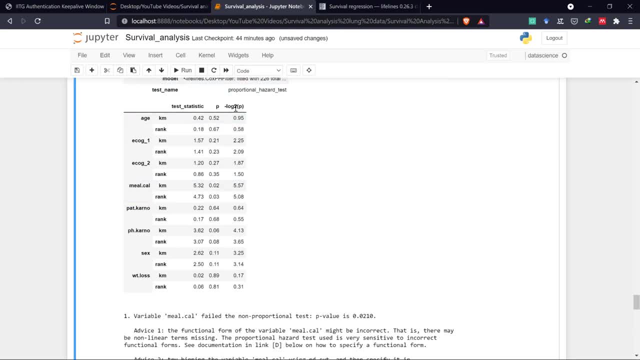 So it gives you this destroyingロstr � właśnie и. And the minus L excuse p. The null hypothesis is that the variable has satisfied the criteria for proportional hazard that the variable satisfy the proportional hazard. The non hypothesis and alternate if I put this with that it does not have to satisfy the 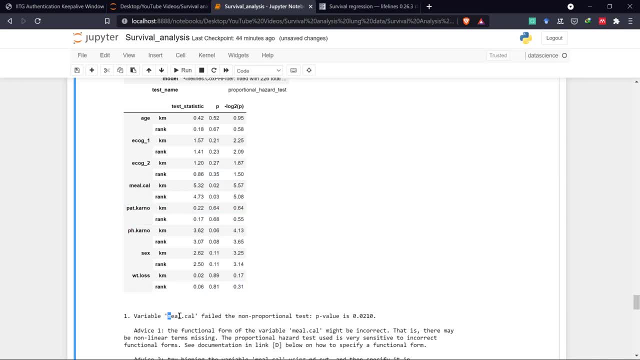 proportional hazard criteria, All the variables. for meal Calorie, The relative 0.001,0.002.. So for meal calorie, the p-value is less than 0.05, it does not satisfy the proportional hazard criteria. Either we can bin this variable into different categories and try again, or different mechanisms. 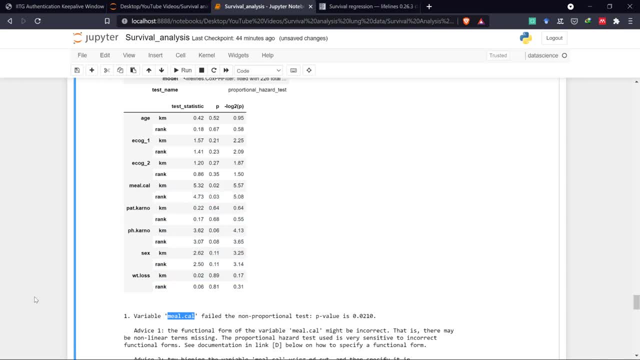 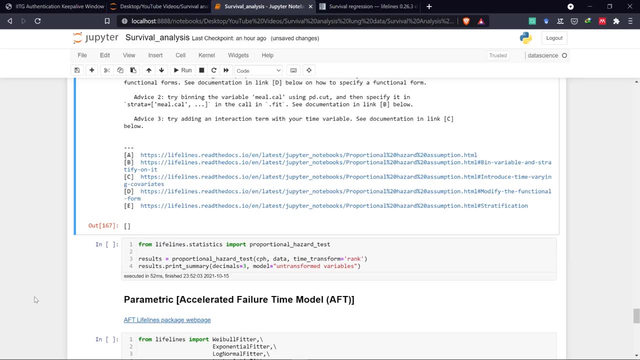 are available to do that. And also we can go for, say, parametric version of the Cox proportional model, But here I am going to use such the parametric models like accelerated or affiliated models. Next, we can also use the lifelines, such as statistics, such as import from the lifelines. 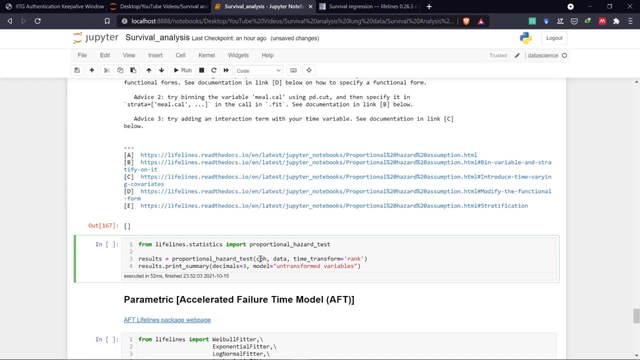 such as statistics, We can import the proportional hazard test. then inside the proportional hazard test we supply the model, object data and time, transform its rank And we will print the up to three decimal place. the summary on transformed variables. 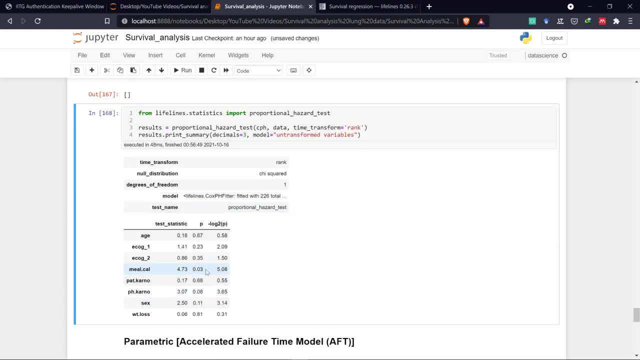 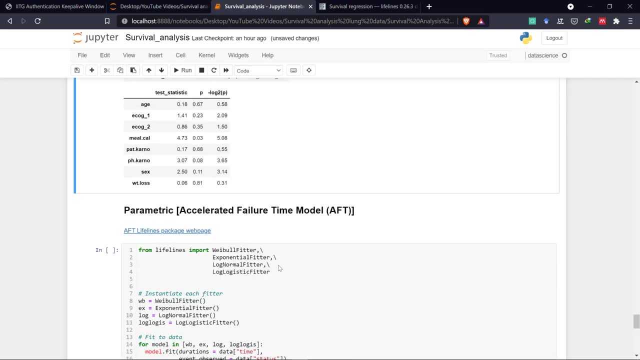 And it will give you the same similar results. that meal calorie is 0.03, less than 0.05, that doesn't satisfy the criteria or fulfill the criteria for 0.05.. So this is the proportional hazard assumption. 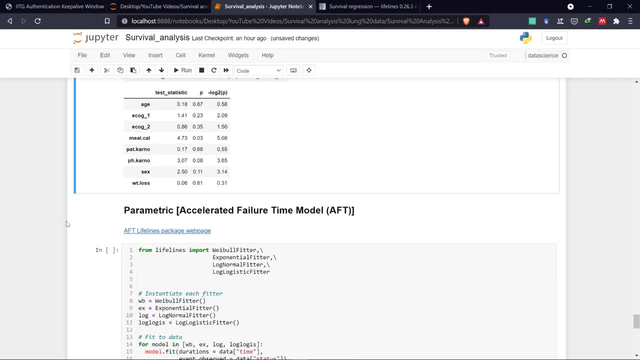 So next is, when proportional hazard assumption criteria does not fulfill for a single variable or large number of variables, then you can go for a parametric version where the we know the distribution of the or assume the distribution, or we already know the distribution. 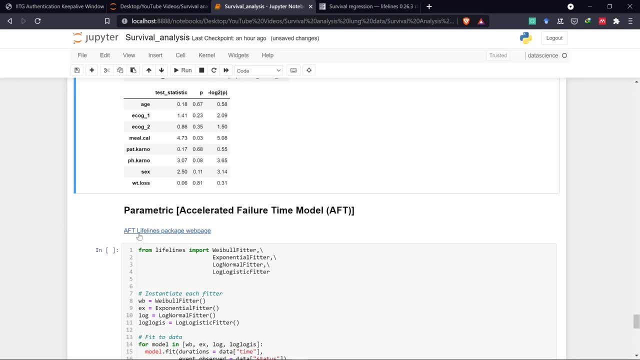 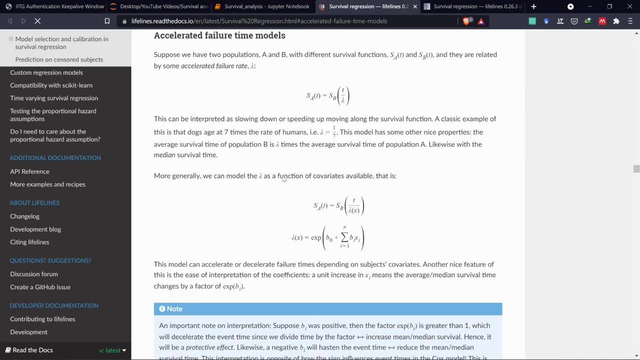 of the outcome variable. So in parametric the AFT- accelerated failure time- model is usually used in for modeling the time-to-event data with covariates like independent variables. covariates mean independent variables And if you go to the AFT in accelerated failure time, this has a good documentation here. 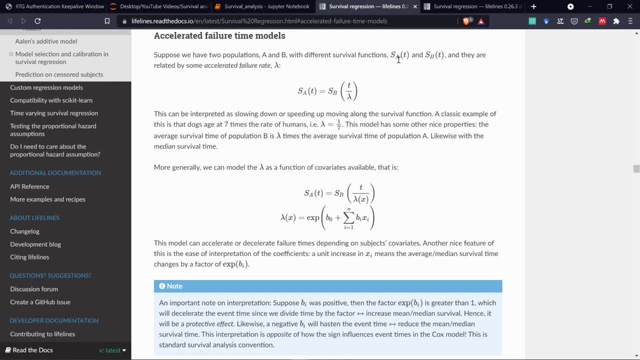 Suppose we have two populations, A and B, with different survival functions- survival A, T and survival B, T- And they are related by some accelerated failure rate, lambda. So SAT is B, SB, T upon lambda, So it is related with H, lambda. 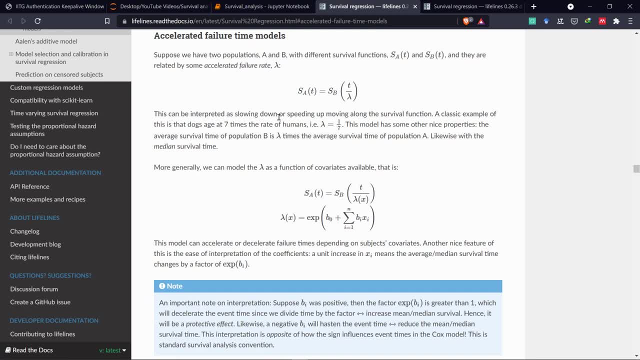 This is the acceleration failure rate. This can be interpreted as swing, slowing down or speeding up, moving along the survival curves, So either accelerating or decelerating, like this. A classic example of this is the, that is, the dog age at seven. dog age at seven times. 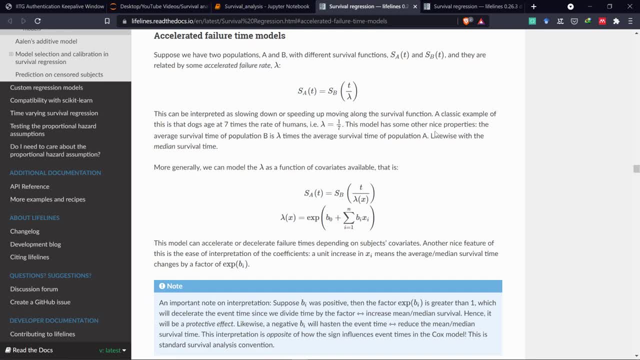 the rate of humans like lambda is 1 by 7.. This model has some other nice properties. The average survival time of population B is lambda times the average survival time of population A, likewise with the median survival time. More generally, we can model lambda as a function of the covariates. 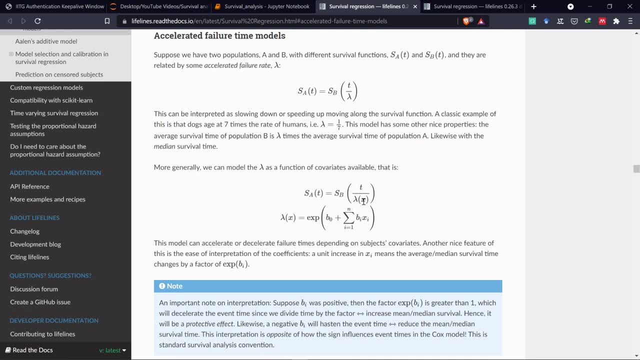 So SAT is SBT and so lambda X. and lambda X can be expressed with the different covariates. like regression, This model can accelerate or decelerate failure times depending on the subject: covariates. Another nice feature of this is the AS of interpretation of the coefficient. 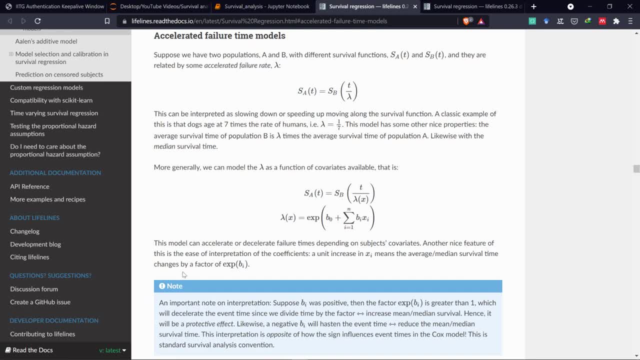 The unit increase in Xi, which means the average of median survival time, changes by a factor of exponential beta. i Okay, So if you exponentiate the coefficient, that is the factor by which it will change. actually An important notice here on the interpretation is that suppose bi was positive, then the 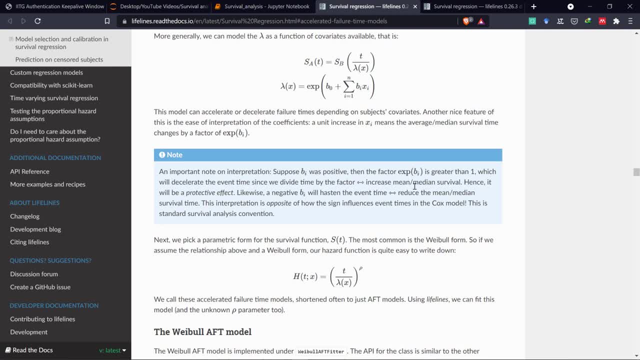 factor exponential bi is greater than 1, which will decelerate the event time. since we divide time by the factor Increases median survival time, Okay, Hence it will be a proactive effect. Likewise, the negative bi will hasten the event time, which reduces the mean or median. 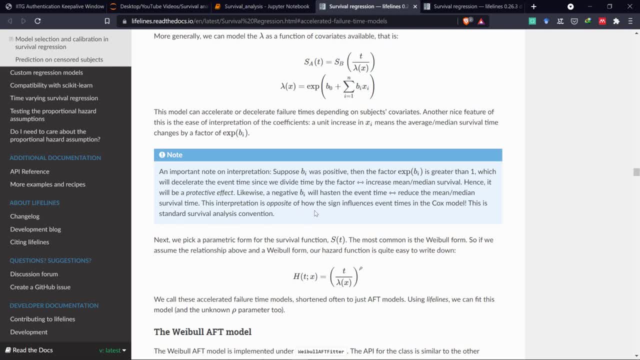 survival time. This interpretation is opposite of how the sign influences the event times in the Cox model. This is a standard survival analysis convention. actually, This is important. note that what is in Cox model? it is quite opposite of that. So let's go to our notebook. 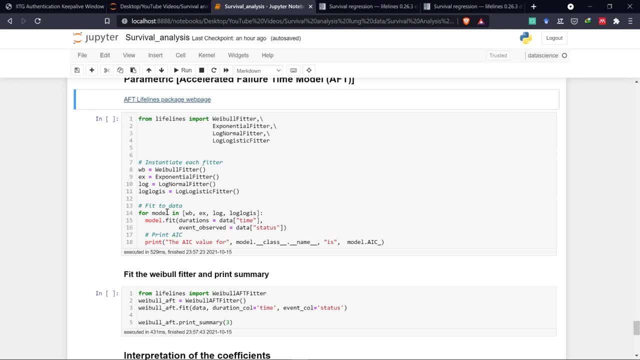 Okay, Okay, Okay, Okay. So the condition isvolleyball: longer than sweet, longer than bi, longer than exponential. All right, So here we look at the code, which does not mention anything. You can see that the variance in this entry is no good right. 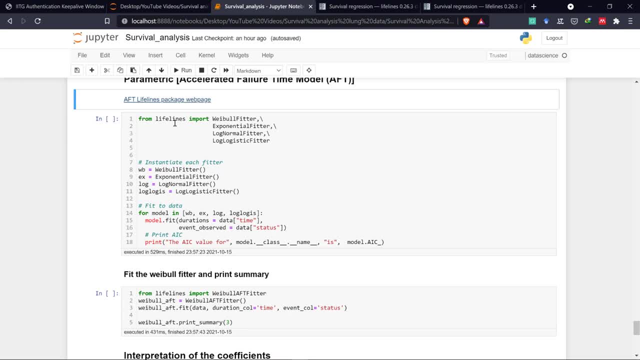 rule, we take the same information as its subject of writing. the variance we use is the variance which of course we can all frame over here, made between: and. then we have to convert it to: yes, it matches, because we already Eunge, but anyway. on the other hand, 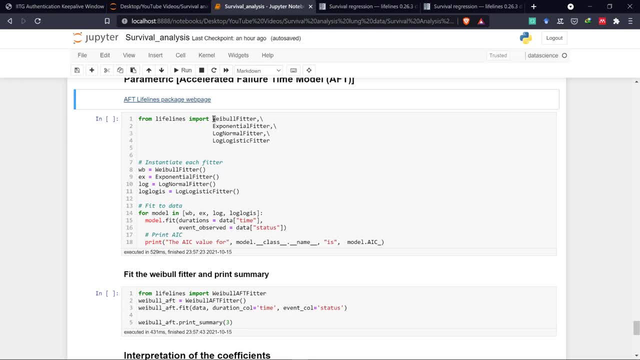 the variance here is normal log logistic. So here I am going to import some common distribution that we will going to fit the Weibull such a fitter exponential distribution, exponential fitter, log normal fitter and log logistic normal. Then we will instantiate as a class and create an object for Weibull exponential log normal. 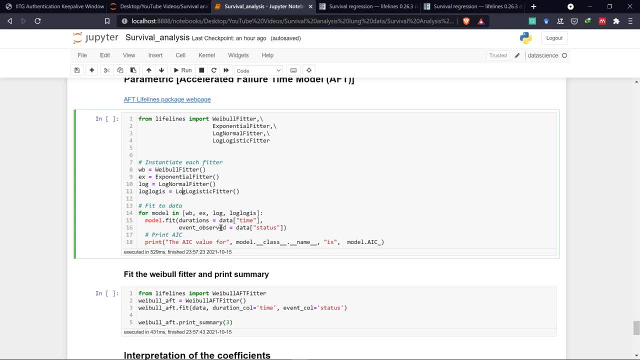 and log logistic. Then we will iterate through each model and then fit the model with its time and status and we print the class model as a name and their AIC values And the lower the AIC values the better the model is. So if we instantiate we can see that the Weibull fitter has 2286.14 lowest AIC value. 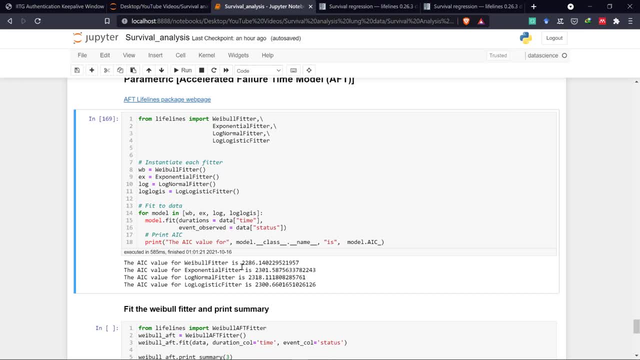 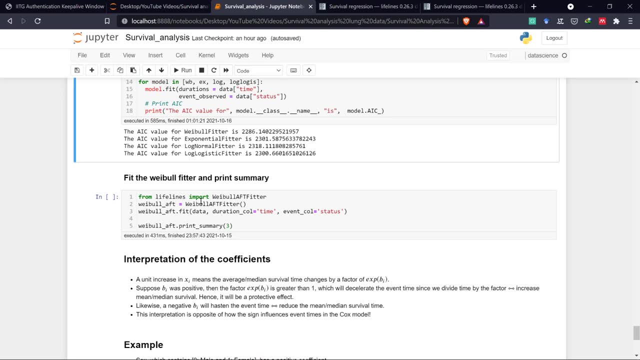 that fits the data best, I guess, So we can use this such a Weibull fitter as our final model. So again, I am taking the importing the Weibull fitter and fitting the model, and now I am printing the summary. 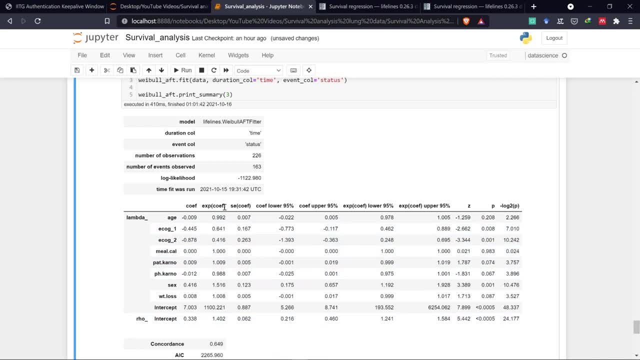 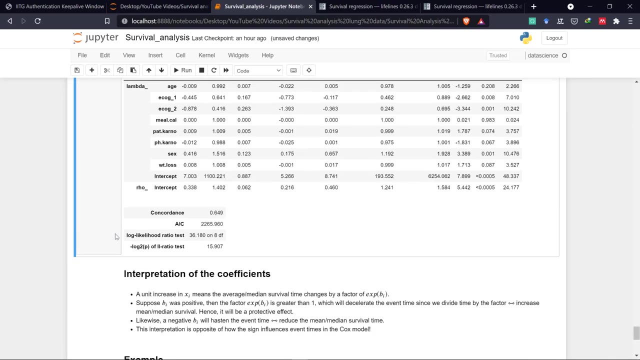 So now I have got this such a coefficients. The exponential coefficient is the not hazard ratio here. It is an acceleration, it is a failure, It is an acceleration factor, or sometimes called as time ratios. So this how we will interpret this: as coefficients or the exponential version of the coefficient. 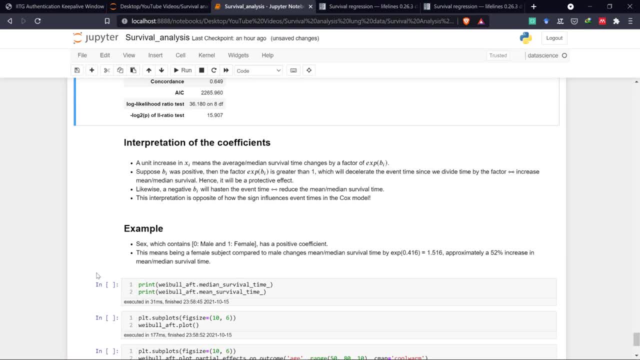 acceleration as factor. So interpretation of the coefficient could be a unit increase. in. xi means the average or median server time changes by factor of exponential vi. Ok, So once vi was positive, then a factor of exponential vi is greater than 1, which will 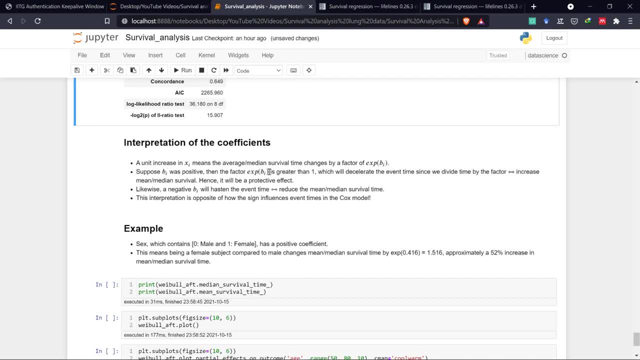 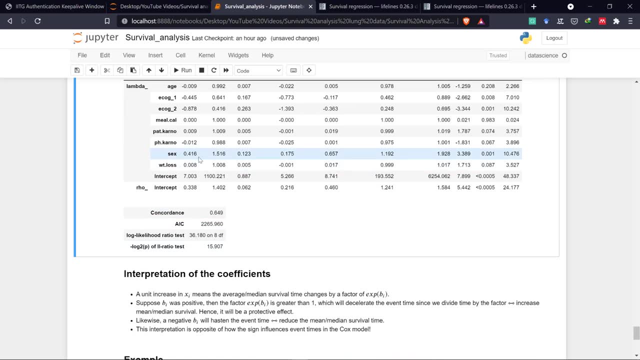 let you decelerate the event time, since we divide time by factor That we already discussed So directly. we can go for the example, For example here, sex having 0.416 positive coefficient with a exponentiated coefficient around 1.516.. 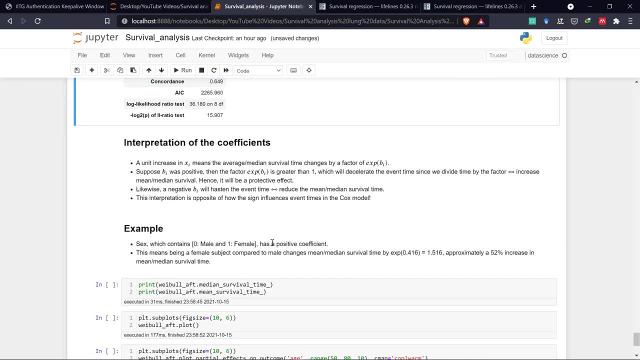 So how we will interpret this? Sex which contains 0 male and 1 female has a positive coefficient. This means being a female subject compared to male. changes mean oblique median is a survival time by area. Ok, So here we can see that sex which contains 0.416 positive coefficient, with a exponentiated